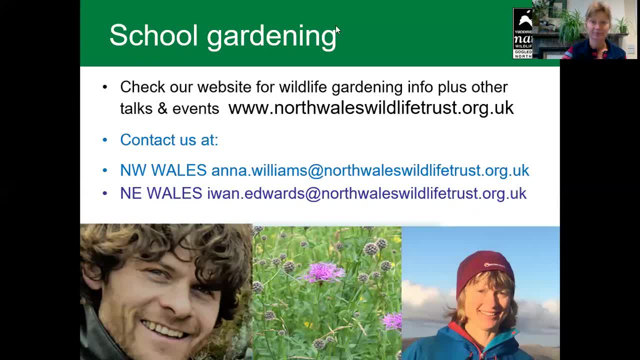 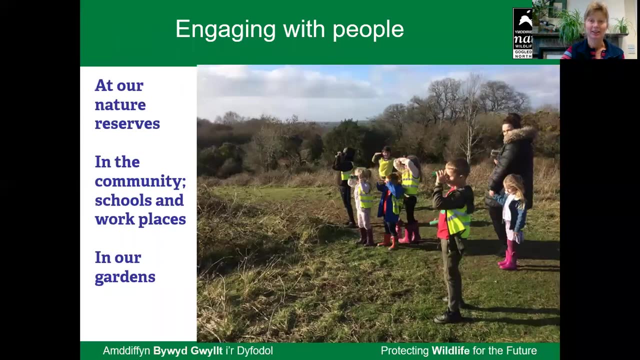 and hedges and so on. A lot of those talks are based- all the examples are based- in schools, So do have a look around, both on our website and our YouTube channel, for more information. Okay, let's get going. You and my work is about engaging with people, and we do it at our nature reserves. So if you want to, 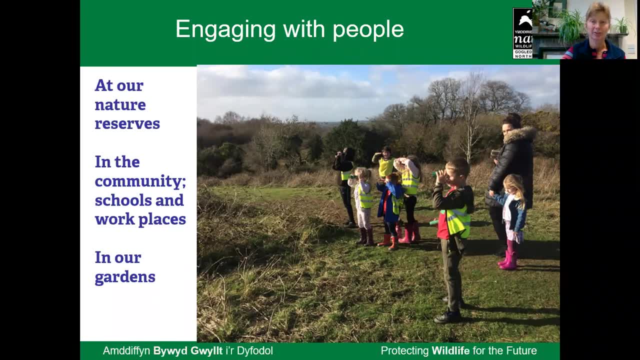 take a school group to our nature reserves. do contact us and you can find out where our reserves are on the website. We also go out in the community schools and we help workplaces, and also I run wildlife gardening project to encourage people- everybody- to do what they can in their own gardens. 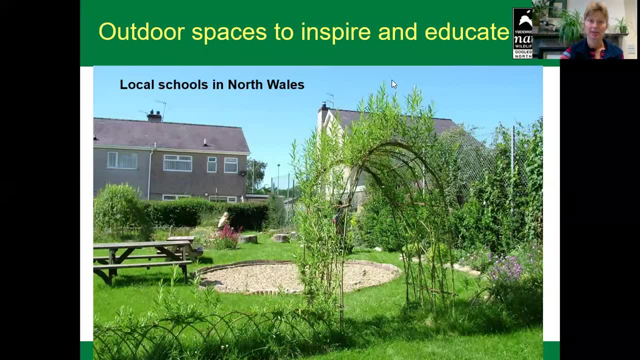 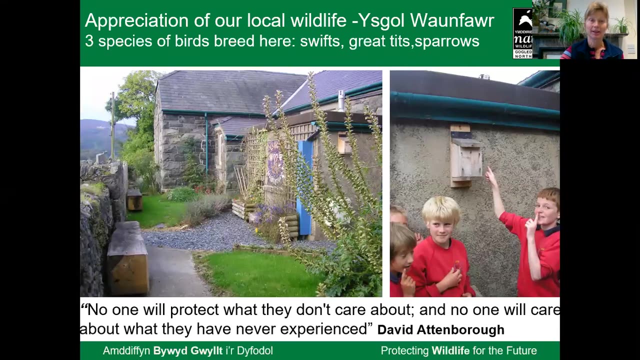 for wildlife. Of course, today I'm going to talk about local schools in North Wales based on work that I've done, and now I'm not going to talk about Ewan's work, but I'm talking about the work in the North West. So it will important part of our work is to win over people's hearts and minds. 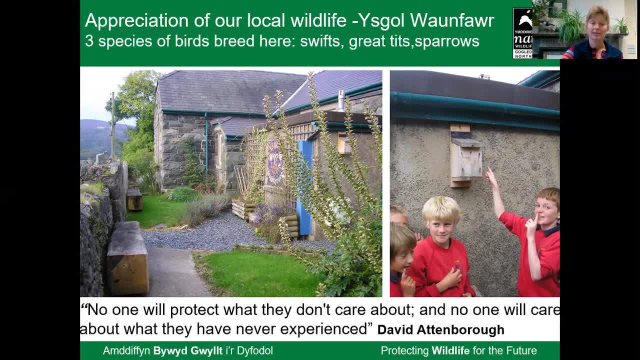 It's not all about creating the habitats but, as David Attenborough says so beautifully there, we really need to have the connection with nature, to care about it and to want to look after it, and I know it's very obvious stating that, but for many children and young people they might not have had the opportunity. 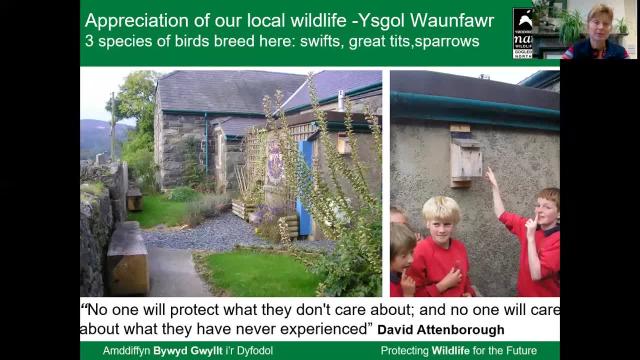 to connect with nature and school grounds is a great opportunity to do this, and the projects don't need to be big. as you can see in this their presentation, and just in that little garden on the photo, we had free birds nesting. So here we have swifts. it's a great experience. you can see the idea behind the bath and then you. 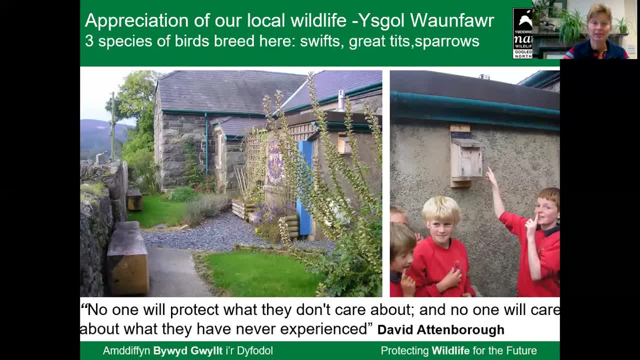 know, the building is completely in this little garden and you can feel the beautiful garden that was built on the ground at the stage. But they are really about the garden. The garden is about in the garden, because the garden is a place that you come and they are. 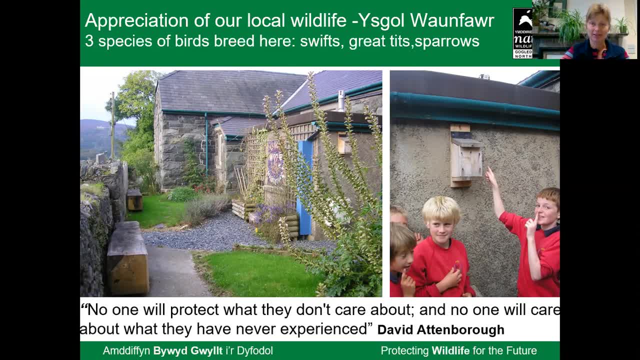 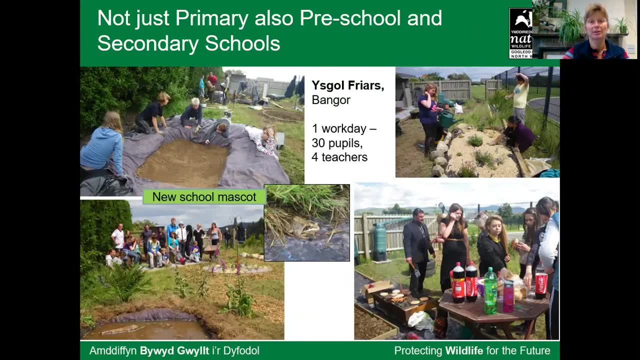 about quality garden and you can look at them and you can see that the garden in the garden and the birds and the flowers in the garden will be a little bit different than the garden in the garden, because if they're durable when they're in the garden, they're likely to be more sustainable. 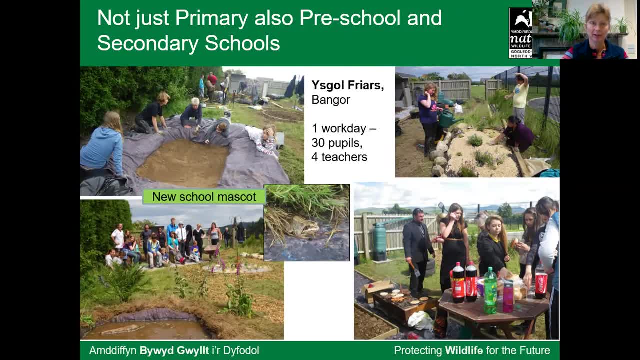 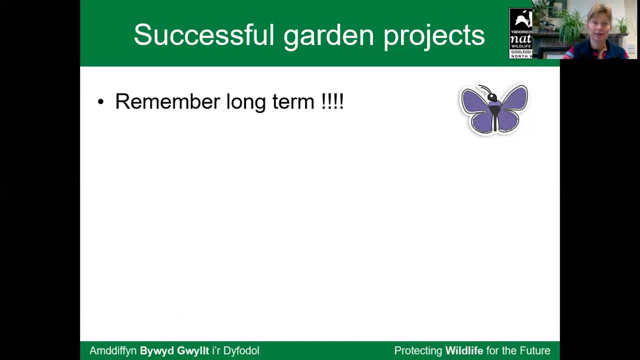 but they don't have to be. They're usually good with water and I'm going to show you what I do with this garden. So I do it for the children projects with us. so I'm just stating a few ideas. I think it's very important to 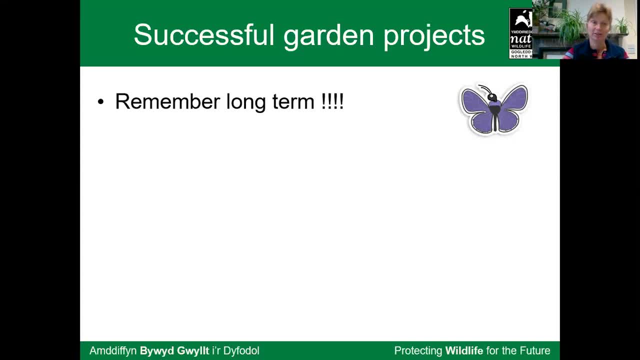 remember that these projects are long-term. once you start a garden, you obviously need to look after it. so it's not just for Christmas, it's for the longer haul. but I think also start small and develop your garden step by step and be realistic with what can be done every year. so it's better to do. 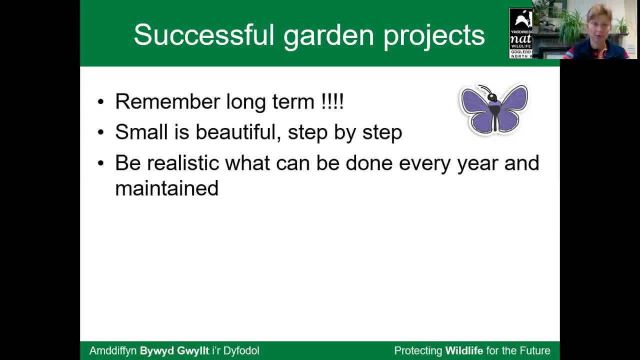 something than have great plans and actually not get around to anything because it's all a little bit too daunting. very importantly, and I'm sure you all agree, it's got to be seen as an asset. it's nothing that's sure. you don't want it to, be sure you want to be. it a place where people want to go and a. 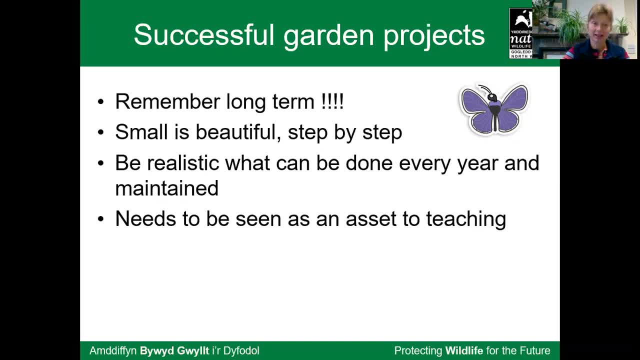 reason to go to school. I've certainly seen projects like that, a school in Colwyn Bay where they, the children, were all green champions in different weeks and the head was telling me that is the first time the children are arriving early to school to water the gardens. so 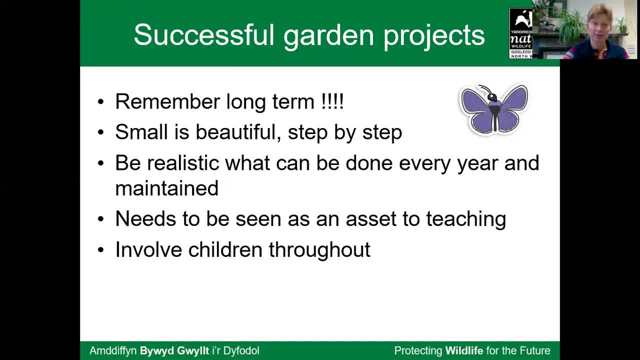 yeah, an asset involved children right the way through. well, for me that's obvious, because I don't think, I don't believe in projects where people are parachuted in to do the garden for us school if you can develop it with the children. because if the process is as 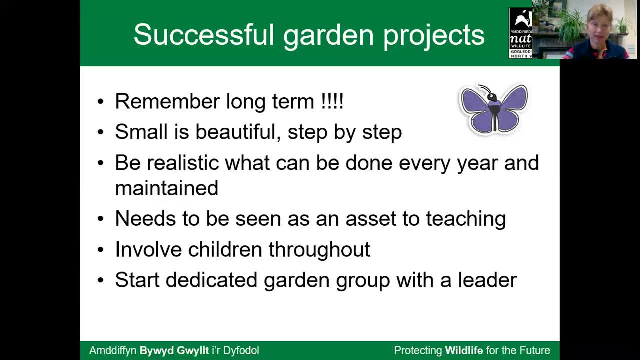 important as the finished result. I think it's, from a management point of view, very important to have a dedicated garden group and then you know who's in charge, who moves the project forward week by week or month by month, depending on your timescape, and in that group you can of. 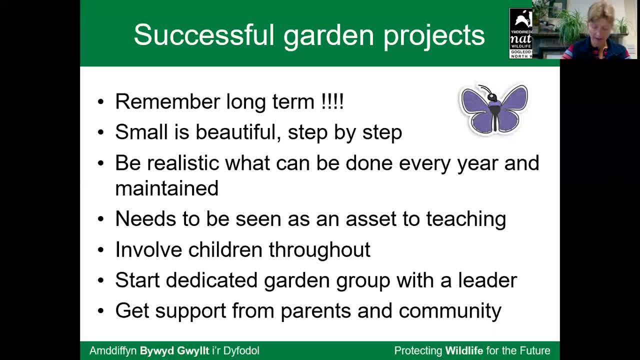 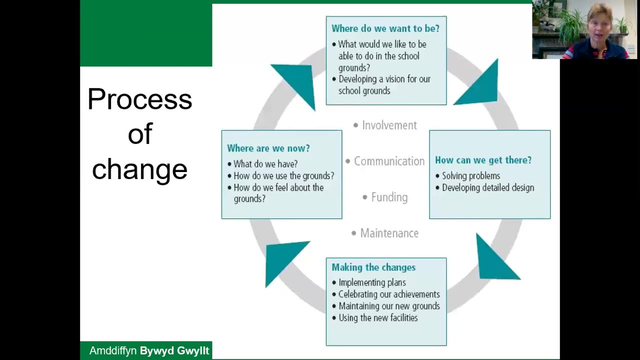 course, get support from the people in the community, and that's how I started a group, actually as a parent helping in a school. don't forget about people outside, because you might very, very well need them. I know it's a bit harder today with COVID and to get other people inside schools, but it can be done. 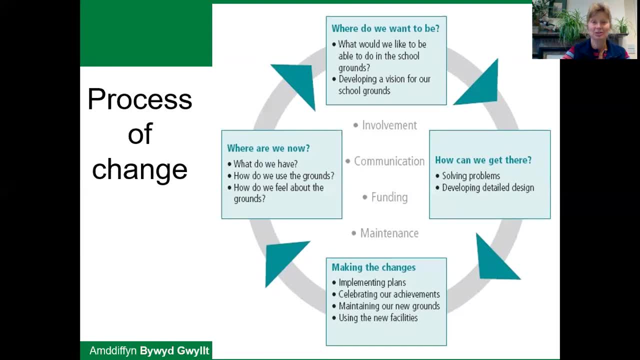 you might have seen different diagrams like this, and this is produced by the learning through landscape organization, for whom I'm also a facilitator, and I'm the facilitator and again, I think, do go through this process. I'm sure you do already. where do we want to be, how are we going to get there and who's? 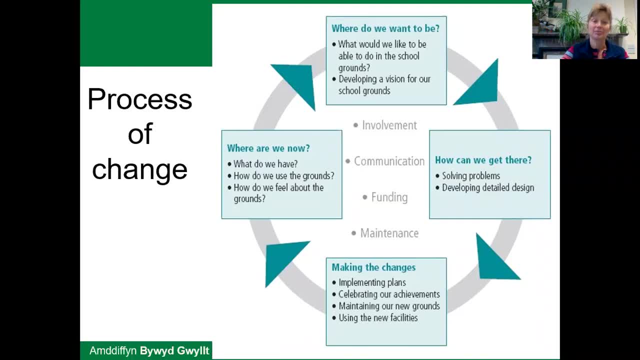 implementing the changes and then, obviously, starting at where we are now. so yeah, do the surveys, do get the children involved with thinking about what we've got at the moment. do the surveys, do the research and do the thinking about what we've got at the moment. do the research and do the. 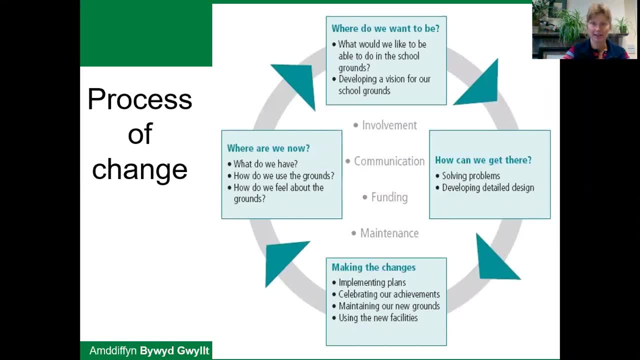 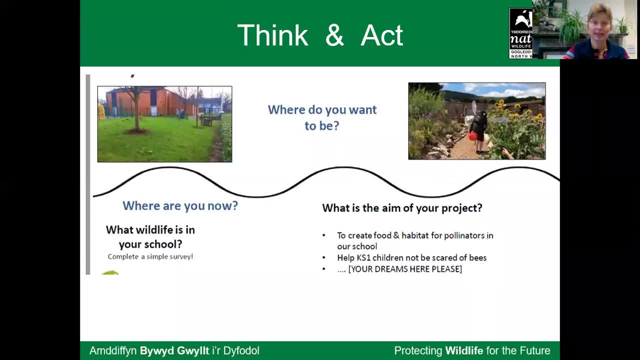 like the yard? what don't they like about it? how could it be better? and then go through the wheel of development. so put in the thinking, but don't stop at the thinking, because that's i can see. that happens as well. make sure you do the action and you can see the transformation of school. 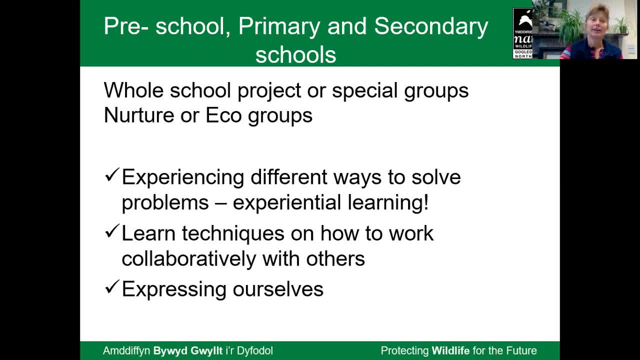 grants through this presentation. um, different schools want to work with different groups. i think it's great if the whole school can be involved. in many rural, slightly smaller schools that's possible. in the larger schools we might work with a year group or there are special groups like nurture groups or eco groups that take a lead. but i think for all people it's a place where you 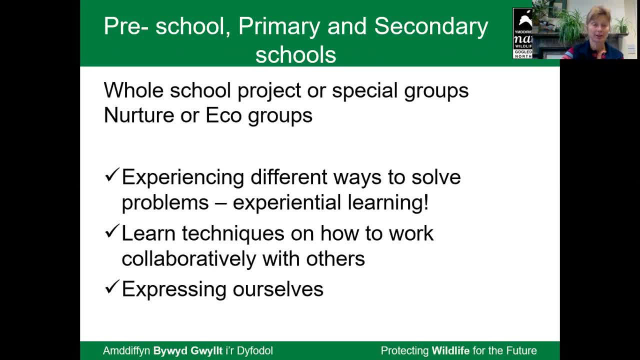 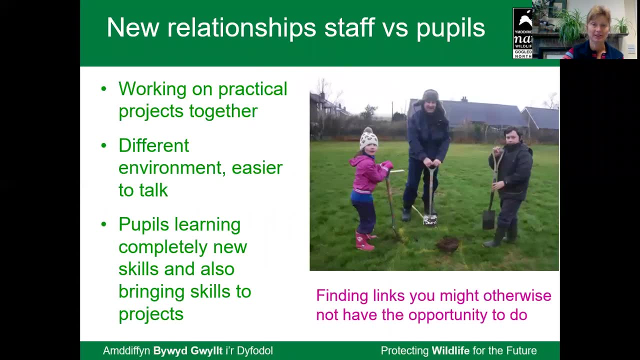 can definitely learn to solve problems in a very different way outside, from inside, from the work you do inside the classroom, and a good way for pupils again to learn how to express themselves, and i will be giving examples of this through the talk. of course, for the staff, it might be an opportunity for you to. 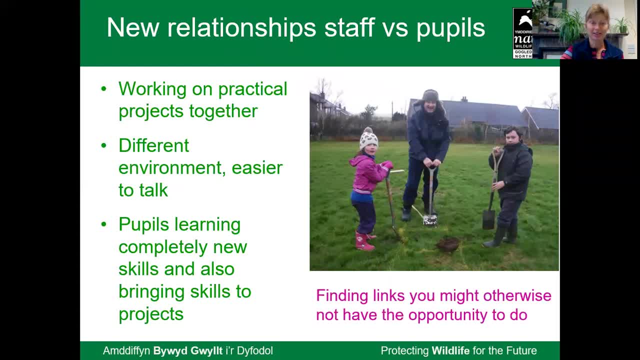 just break some barriers. doing practical work is brilliant for opening new relationships in a way, and i found that when i come in the children are very eager to talk. i hear all the school gossip and they also can bring skills from home that they know things, that they know things that they have. 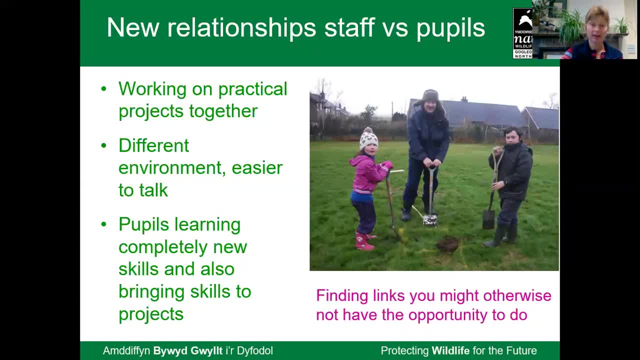 learned outside of schools. and here's the headmaster getting to grips with planting some apple trees up in ross godwin. i know his move now, but i think it's good for the teaching staff to go out and also get the hands dirty and get involved with this project. so today i'm going to go through different 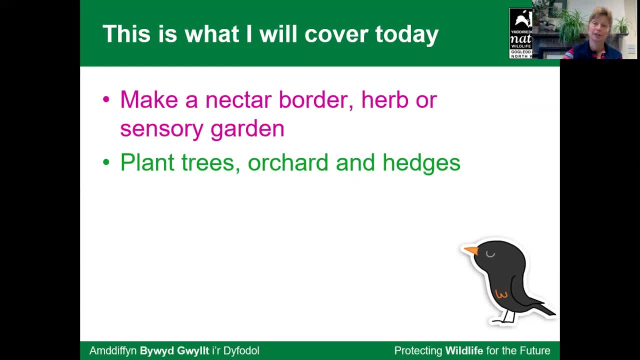 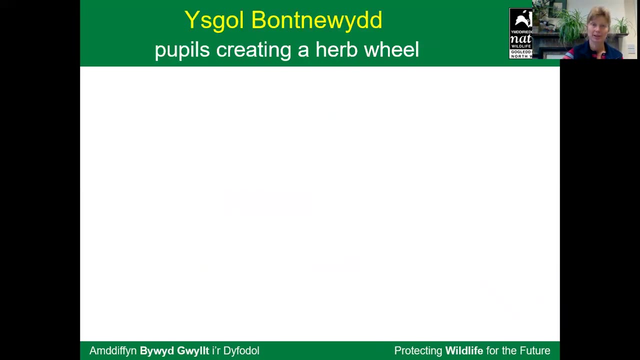 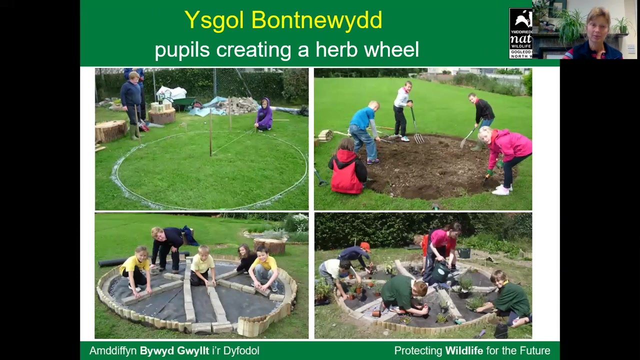 different areas of outdoor development: borders, trees, orgies and hedges, meadows, velo dames, fruit growing- and then just showing different projects. so let's get started. so in bond normal they were doing a hub wheel and we had a very small budget on this, probably not much more than 100 pounds. actually the bricks that you see there. they move them all the way down. nowadays we've been able to the the route has been added, so that means that i think the更or Cowan Bay orthopedic thing can. 90% of of this is not in an ideal condition, not the difference between how it works, but looking for. 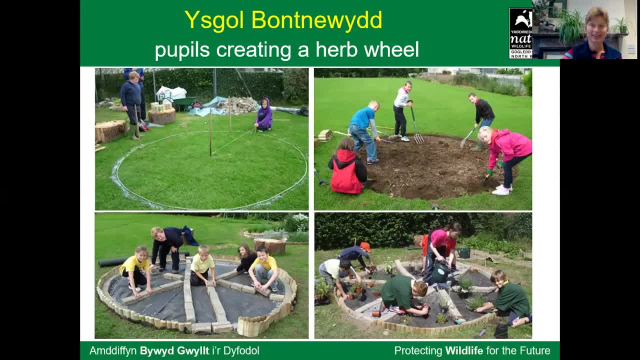 bricks that you see there. they were secondhand from Carnarvon Square. Anyway, back to the pupils Developing even a simple thing like a herb wheel. Of course you need to design it and then we need to work out how big are we going to make this circle? It's really interesting doing practical. 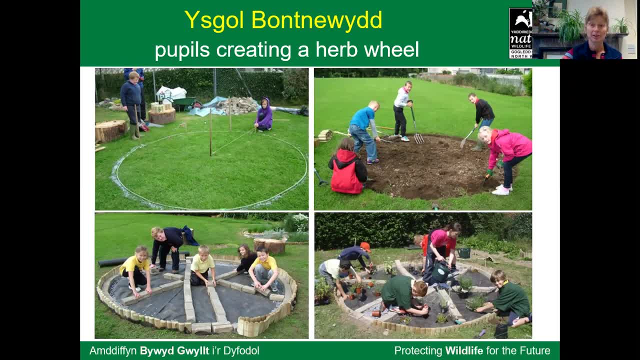 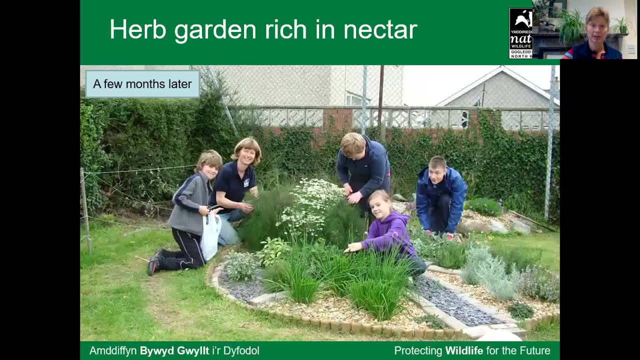 maths, and how do we create a circle and mark it out accurately. Then we're dividing it into segments and again, with a bit of inspiration and imagination, you could do lots of work here in IT as well, and drawing and technology, of course. Then we've got planting and you have a resource. 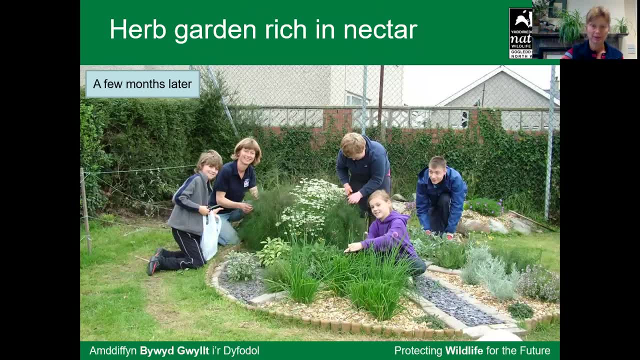 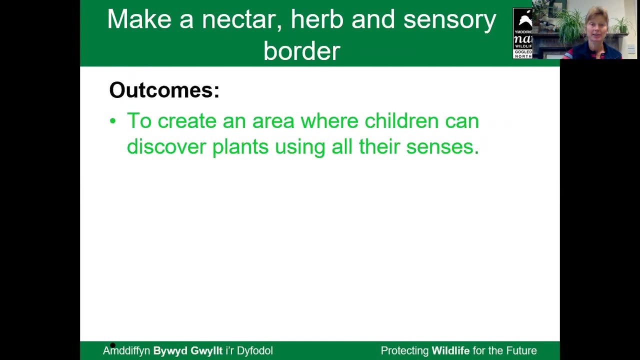 herbs for the school and also herbs to take home if they want. All herbs do best if you do prune them regularly. So I think the boy there he's cutting some chives. So for each of this area of habitat we can write down the outcomes. 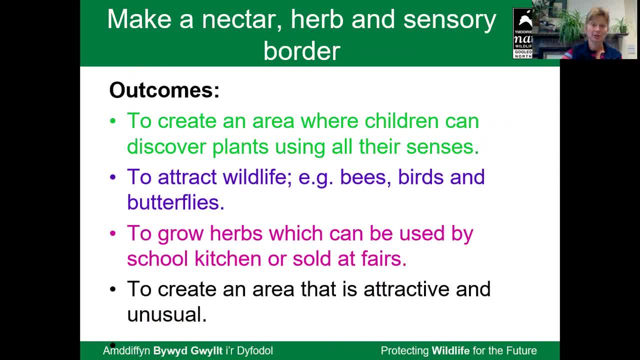 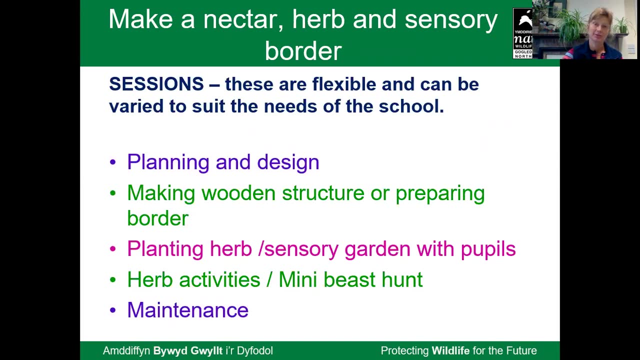 and I won't go through them one by one, but this is something I suppose you do need to show and think about. show to management and think about yourselves. Why are we doing it? What do we want to achieve? And then sessions. I have these sort of sessions link the curriculum for each one of the different. 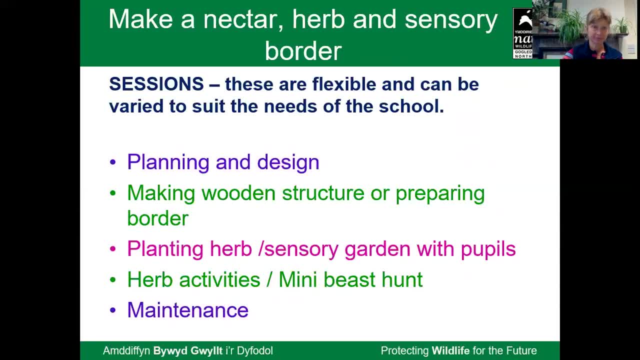 projects. So if you want them, I can send them to you later. And of course, these sessions can be done by the schools entirely yourself. or if you want to bring in an outside body like us, the Wildlife Trust, we can do it in collaboration with you. I think that can work very well. 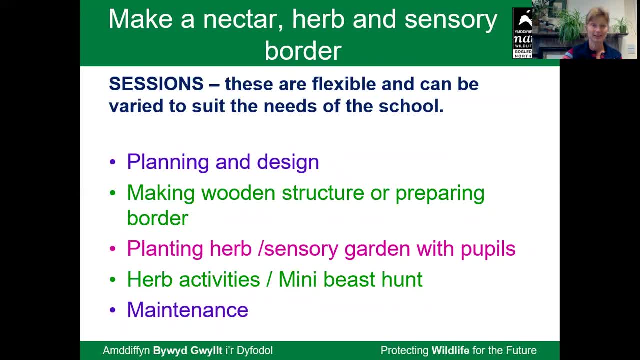 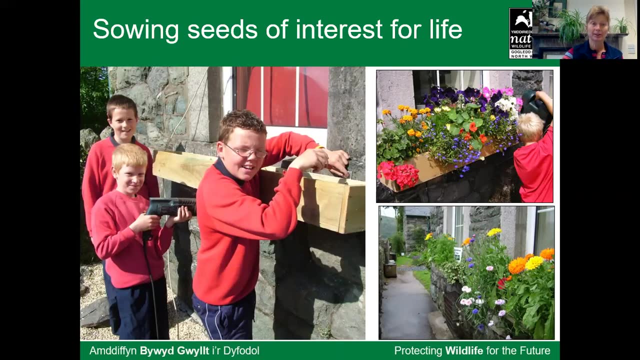 But the school definitely has to take ownership of the garden and the school is the main driver Because at the end of the day, you are there to do the maintenance and the teaching outside. So in our school gardens it's not only about learning topic to topic, I think it's. 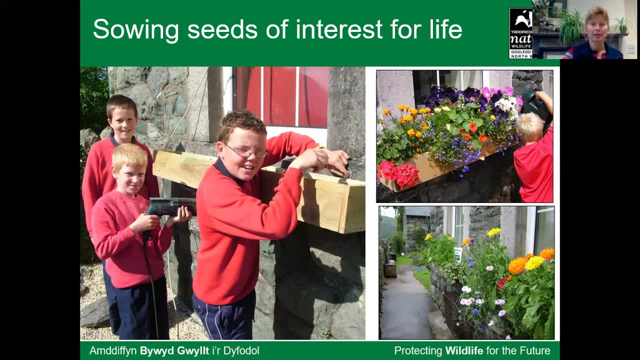 deeper than that. It goes a lot deeper and hopefully we can give some of the pupils anyway interests outside of school and the natural world is vast and many people do get inspiration. Some of our best naturalists have got inspired at school by people coming in or giving a talk or 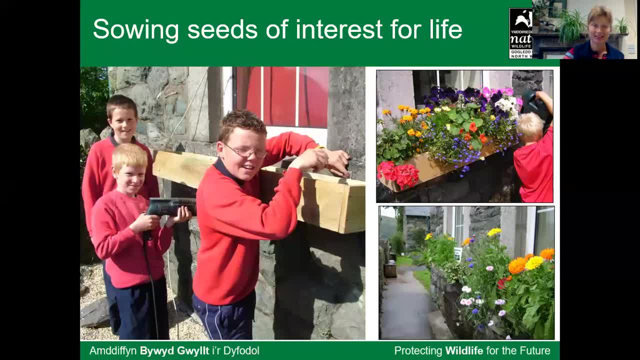 whatever it is, And I know the lad here in the middle on the left hand photo. he is now a tree surgeon And Arwell was very inspired by the school gardening project we did in Weinwald. He was so keen he had to start a school garden at home And his mother has told me that he's now. 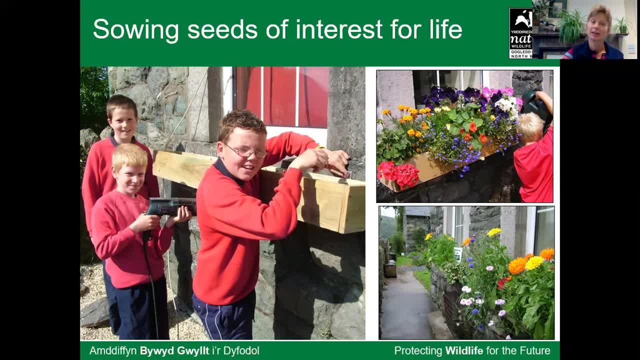 really happy in his work and he loves going to work every day And the school garden had a big influence on his choice of career. I also know that the boy in the front there, Thomas Perry, he had a good day and the headmistress at the end of this day planting. 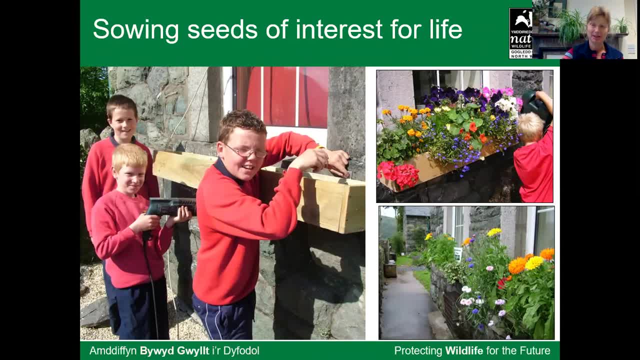 the window boxes. She came out with two bits of paper, very excited, shaking them about together, And I was going what's on, What's up? And she was telling me how Thomas had written more than he's ever done in school before. So suddenly, from this day, which motivated him and inspired him. 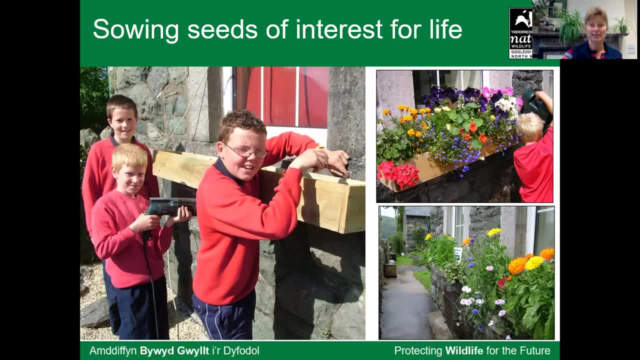 he had a lot to write about. So stories like that that are important, And of course in these window boxes- they'd already made them first of all themselves. You can grow herbs or just nectar plants, And I think the children we had raised most of those. 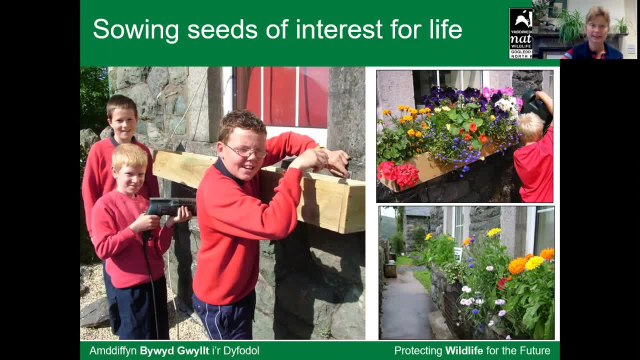 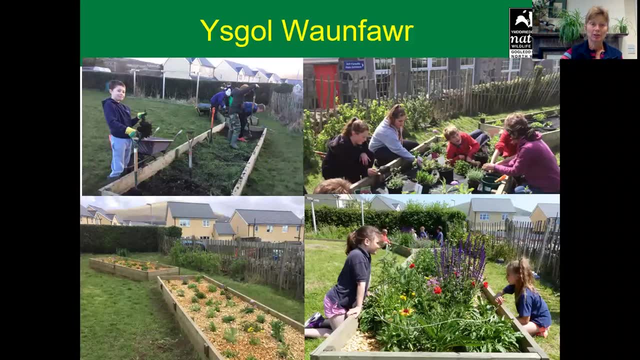 from seed, but you can always buy them. Nothing wrong with that. So in Weinwald again they were involved in a pollination project and here returning some beds that used to grow vegetables in. they were turning them into nectar border And the 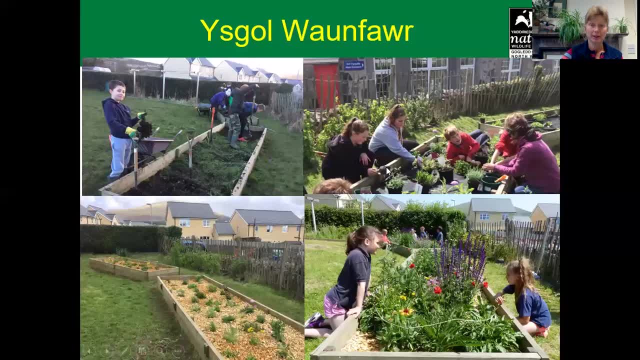 children were doing a survey So I found with schools it's very good to plant through weed membrane. It's a bit awkward. We lay the plants out, try and maybe mark out where the plants are going, dig holes and then put it on again and then plant through the membrane, Put some gravel on. 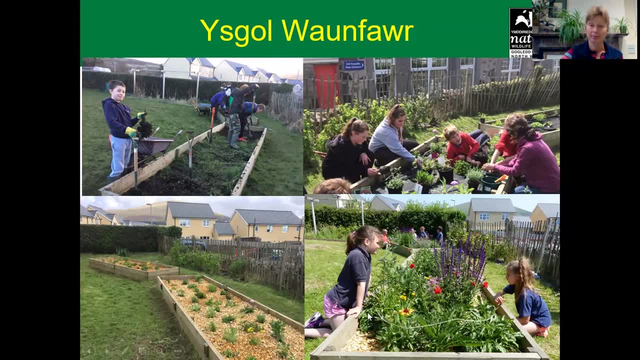 which actually the butterflies really like to bask on before the plants take over and the bed is full of them. So here, the children on the right. they're doing a survey, looking at how many bees and bumblebees are coming today. Nectar borders, That's probably the best way to do it. 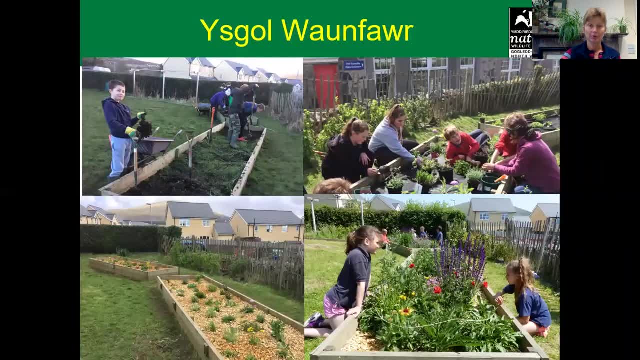 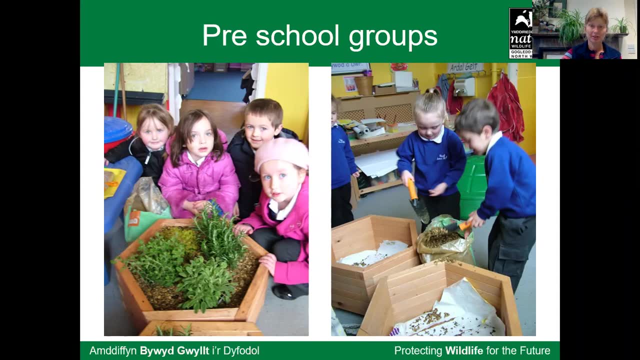 Part of this pollination project. We can work with different ages and, of course, herb gardens are great for the little ones- Sensory gardens: you can touch it, you can feel it and you can eat them, So let them get messy and involved as well. You all know about the new curriculum. 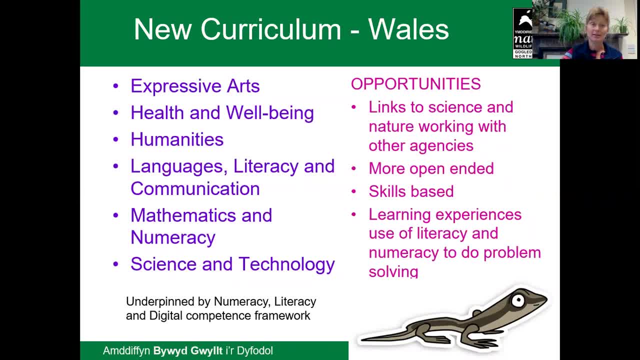 but for those people who are not teachers, these are the six main learning areas, So I won't go through them. You can read them yourselves. It's obviously based on similar ideas as before, but having talked to a few heads of schools, they seem to. 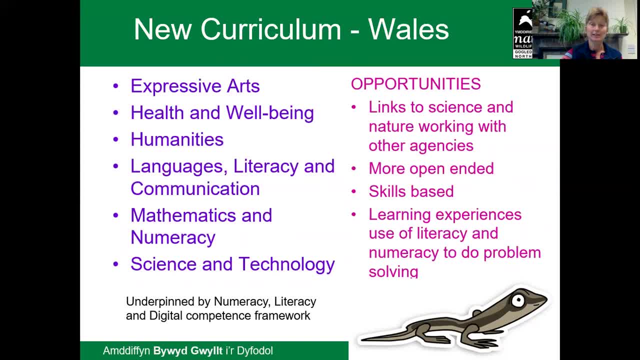 think that with a new curriculum it will be easier to do the school gardening project, linking it across different subjects, more open-ended and very much skills-based. So in these projects I think you will be able to have learning experiences using literacy and numeracy. 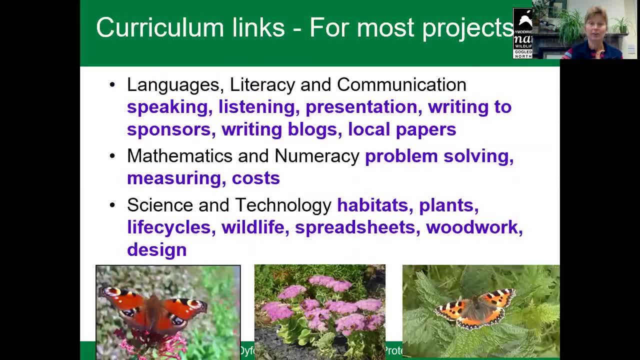 to do the problem solving. So, as far as curriculum links goes, for nearly everything you'll involve languages, speaking, listening, presentations like the one I'm doing now, And for many projects we've written to local businesses and people's often been successful as well. Blogs, writing to. 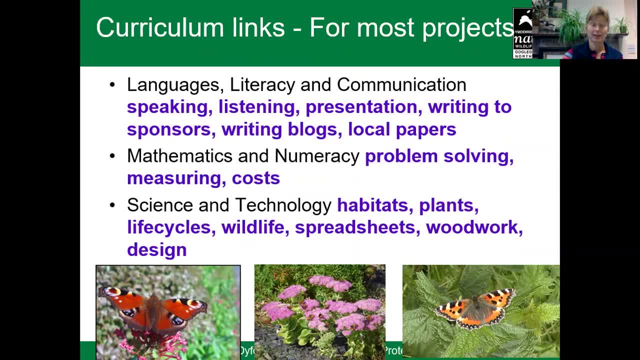 papers. of course there's a lot in maths And science. maybe is the topic that most people think about, but there is a lot more than science to be done out in the garden And for many projects I've done, I know teachers have said that that is the most I've heard that pupil talk. Oh, one little. 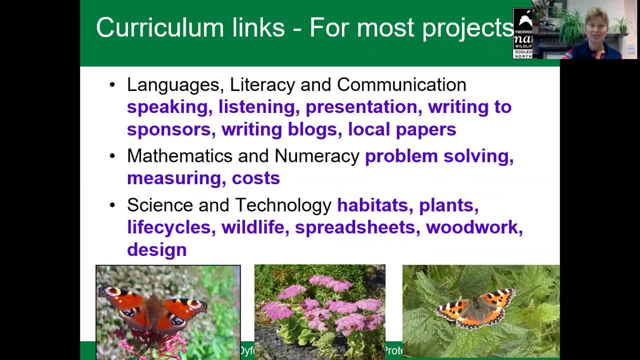 story. It was very touching. We'd done a bug hunt and the teacher said to me that's the most I've heard from this little pupil all term and that was in an afternoon of doing a backhand, actually at our own garden here. so 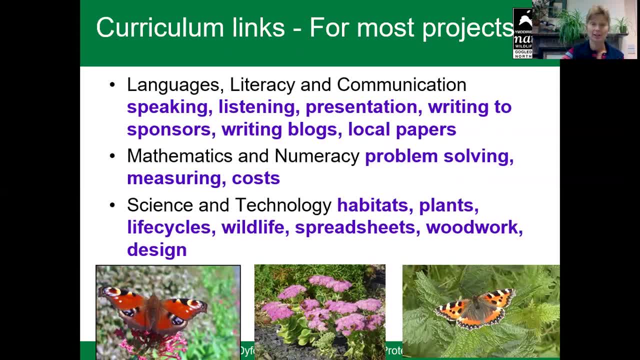 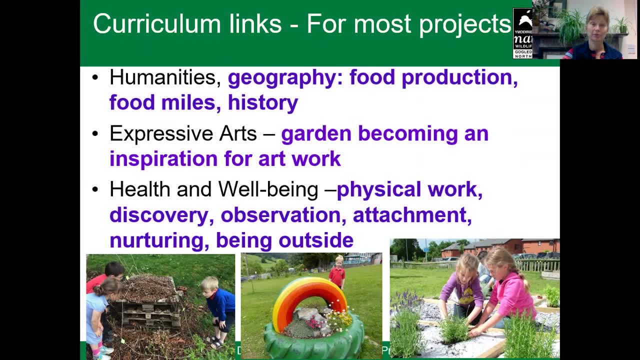 i think doing something different sometimes brings out different sides of pupils. of course, we can cover even subjects like geography, food production, food miles. that's very interesting and comparing it with local production and especially, uh, poignant in this time, and i think there is much more interest in growing and eating local food history. 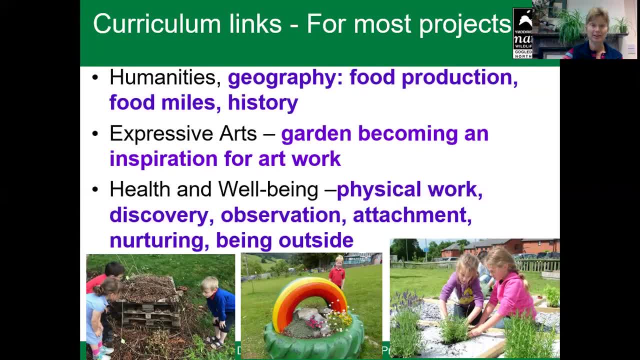 what did they grow during the war? and there's a few schools that have done the dig for victory plantings and so on, and it's not i mean history all only going back to grandparents. very often the grandparents are actually the, the family that the children have done gardening with. 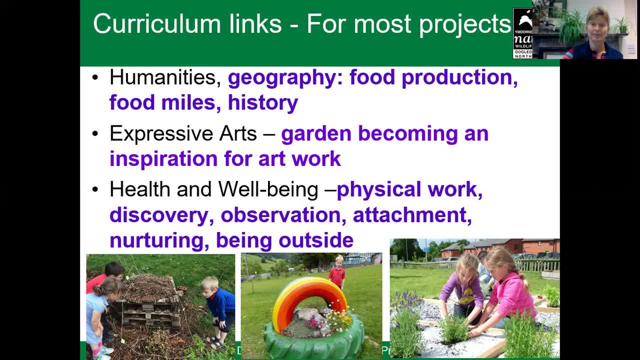 at home. so the grandparents are brilliant resource and some of them do also come in and help at school. well, that was all pre-covered, but hopefully after there were some grandparents who might like to get involved. art: i think it's fantastic. the garden: some schools they use the garden for inspiration and you can do art in all different 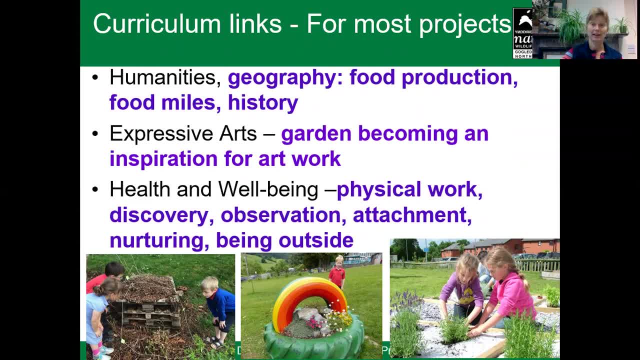 materials, obviously drawing clay, photography. there's a lot to do, and i think it's also. it's a resource that allows us to you to observe the seasons, and if you are good at keeping a diary or a blog, it's really interesting to go out and take a photograph. the same view right through the year, and then the children. 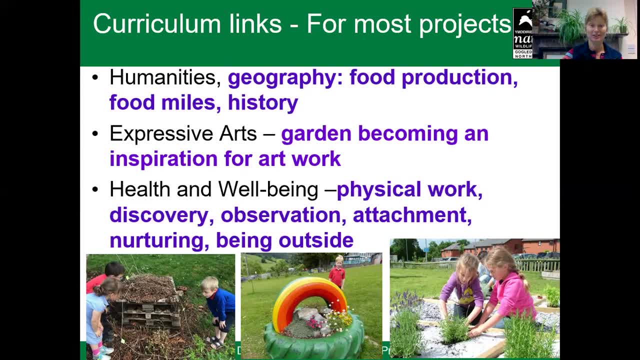 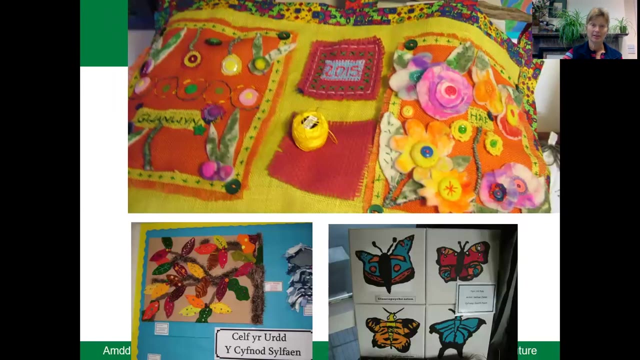 can have their own phenology studies, studies of the seasons in their own garden. the health and well-being i can't stress enough, and i think just being outside uh distresses all of us. observation and discovery of the natural world has definitely also improved people's mental health, so i think all of those are very important. some examples of some artwork based on: 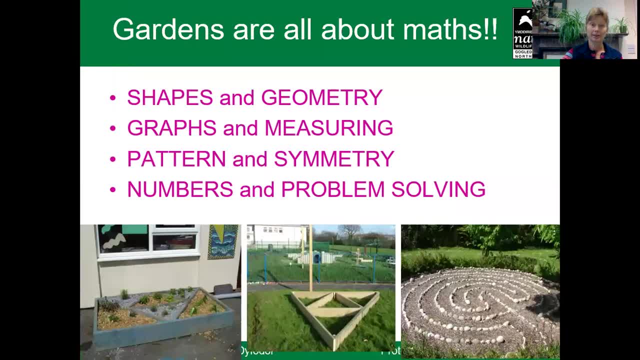 the garden- unsurprisingly maybe, i having done this work- uh, gardens, there's a lot of maps in the garden and all about the shape of the garden and the opportunities of the absolument, and then all of these will be laid out and i think it's really interesting to see what. 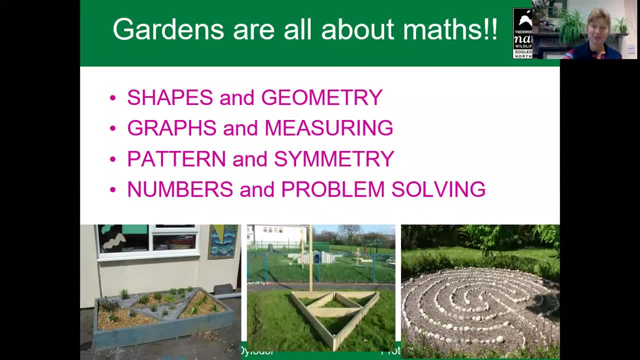 maybe i haven't done this work. uh, gardens, there's a lot of maps in the garden and all about the shape. I can go into this and I can post a little file with more work that you can be done in school, based on garden: all the different mathematical exercises you. 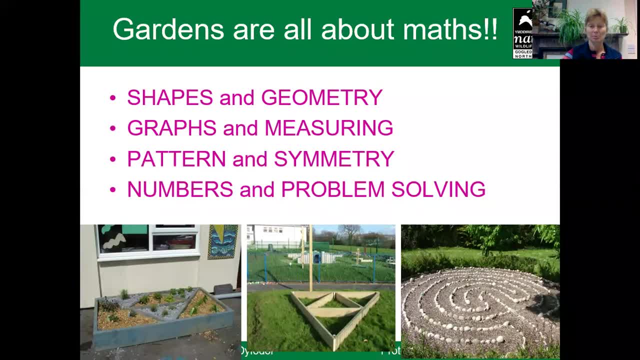 can do. so. there's a lot, yeah, numbers, problem-solving, area measurements and, I think for many people, again using a tape measure, actually realizing what is a meter? how long is it? one school? it was really good we had a meter sticks and we could just play around with them and create different shapes, and then they 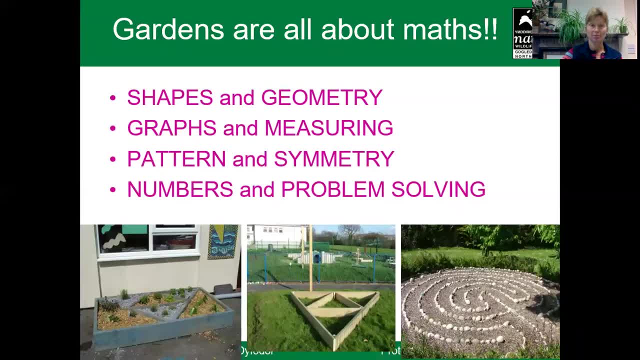 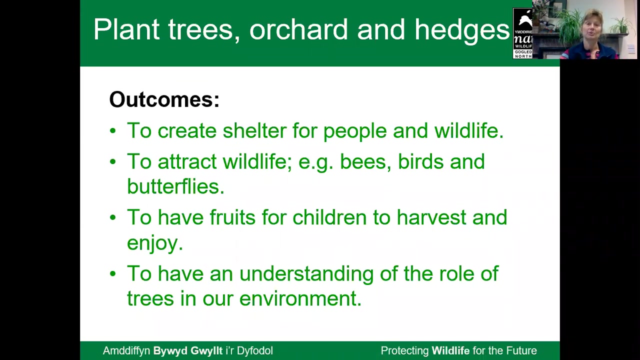 could see by increasing the circumference how much bigger the area became, etc. etc. so doing something practically it's great and they can learn about Pythagoras and Fibonacci and all the different can do lots of different problem-solving. so from I talked about nectar borders on to the trees and trees, obviously it's. 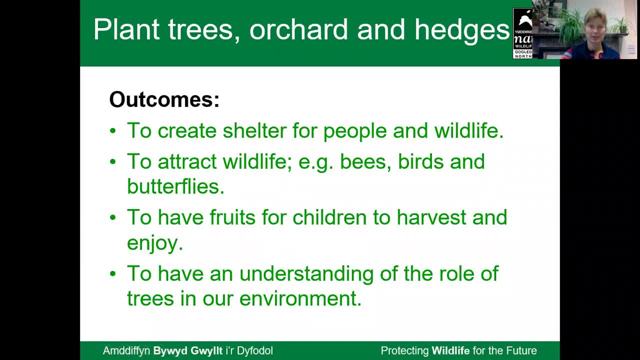 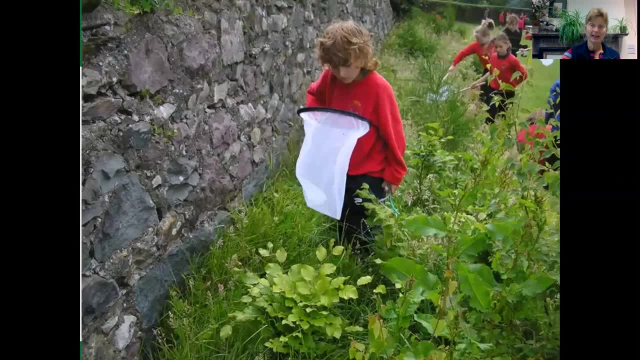 hugely important in any garden for very obvious reasons, and I will just take you through some examples of work we've done with tree planting. hedges are great and if you can only do one thing- even a perimeter hedge where you leave the grass to grow long- it's an excellent resource for things like bug hunts. 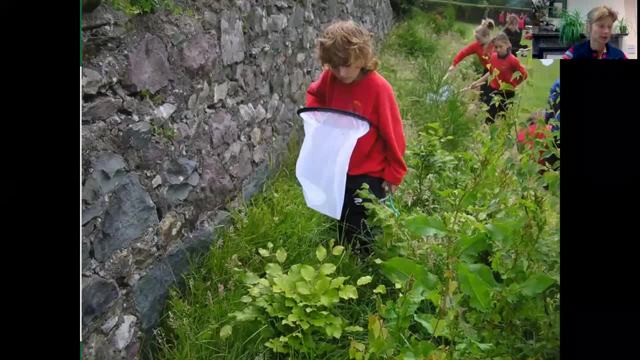 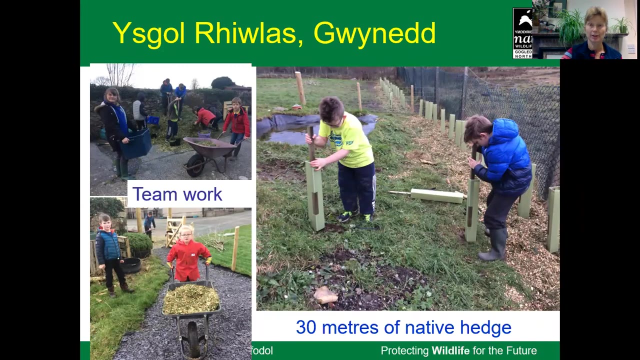 you here. we spent a happy afternoon looking for bugs, and there was so much to find. you don't need to be an expert to do these things with the pupils. you can learn together with them. a long hedge in Rulas, which is a very exposed school garden, so we needed protection, and they also wanted somewhere for wildlife to 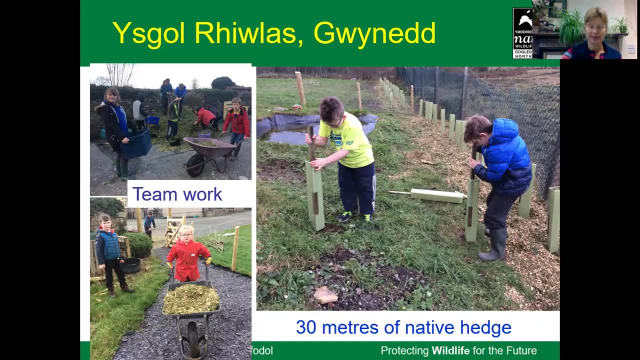 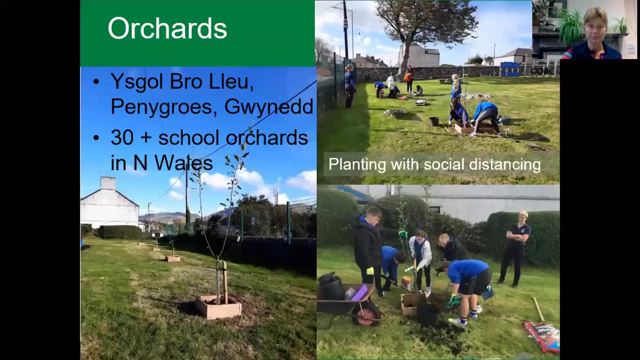 nest. many schools have these ugly fences and double road hedge like this will give fantastic covering years to come. I've been out this autumn planting some orchards. this is standing penny growths. we managed- you'll see a little film later- we managed- to plant eight apple trees in the school garden. 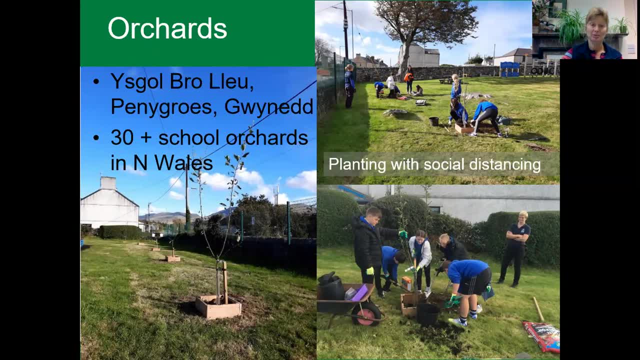 Apple trees is also a very good tree to plant in any school. it obviously gives something back to you and it's very good for pollinators. so think through your intentions and then you can continue to plant more, because that's what you want to do for a good school garden. 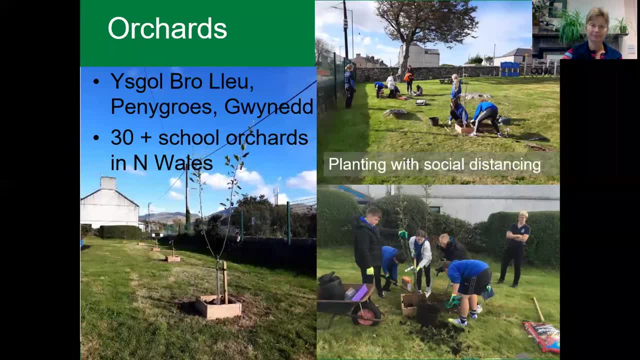 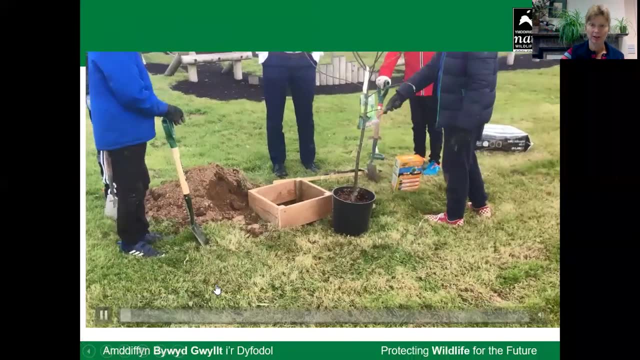 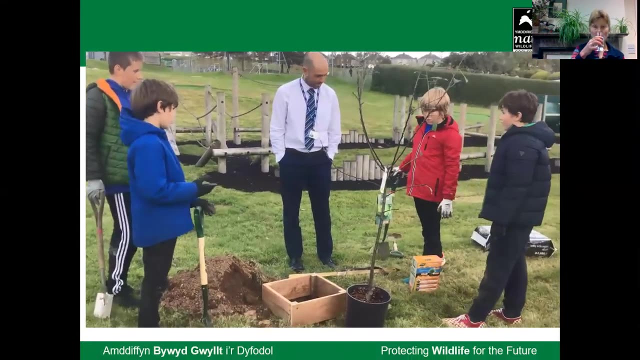 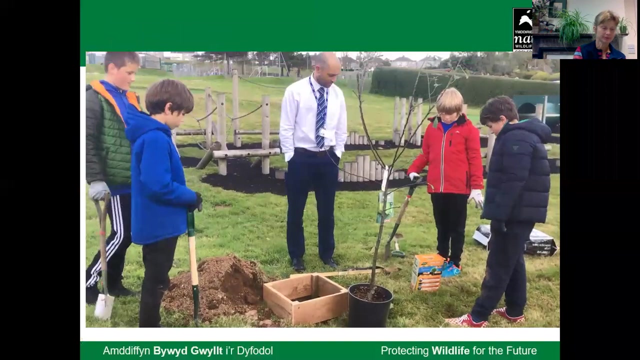 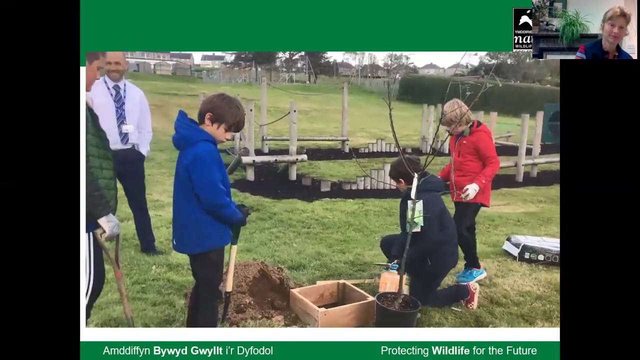 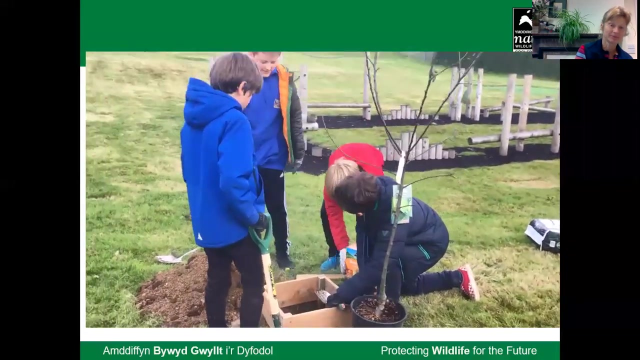 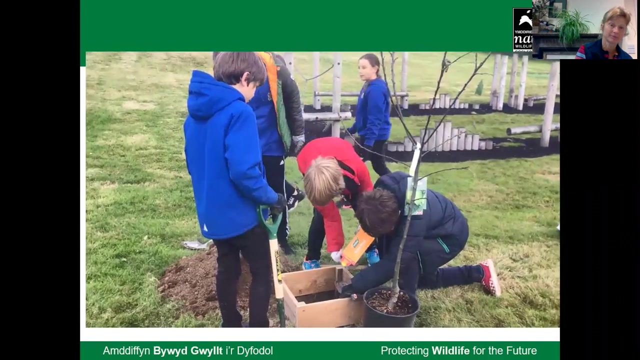 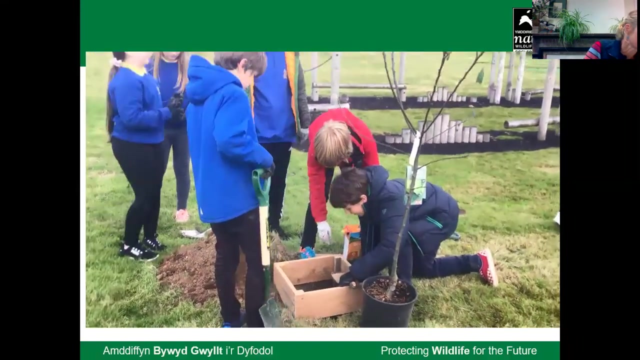 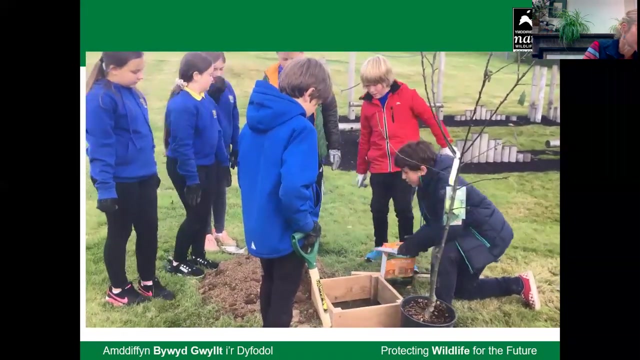 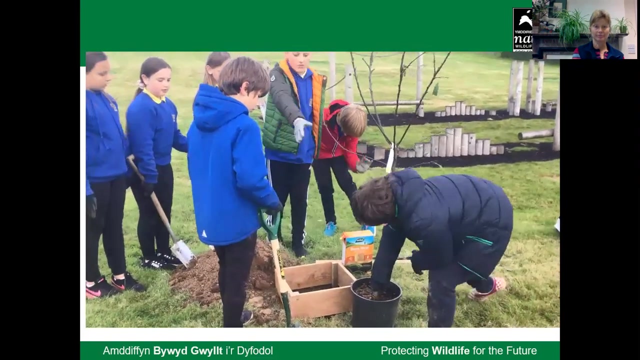 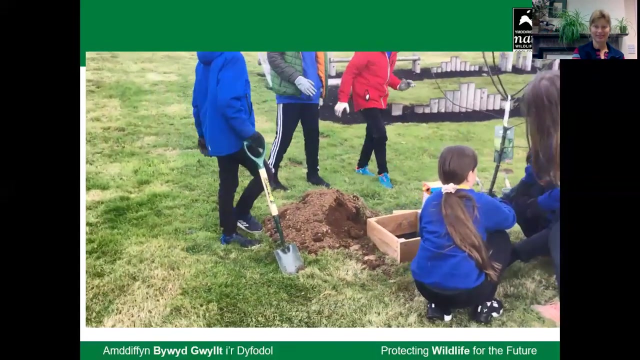 fruit trees. if you're about to plant any trees. oh yeah, here's the film, so let's. the audio is not very good, but that doesn't matter. I just give you two minutes to have a look at this film. you, the lad, is just saying that now we need more than one person taking the tree out. 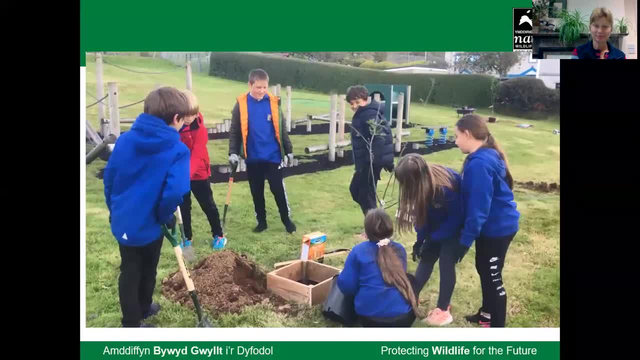 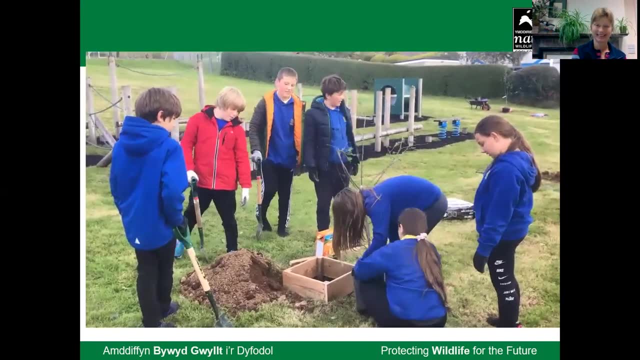 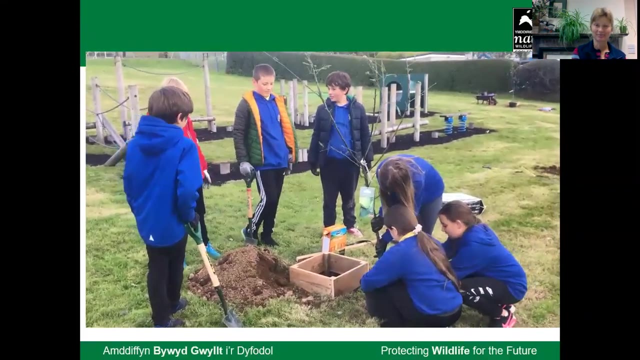 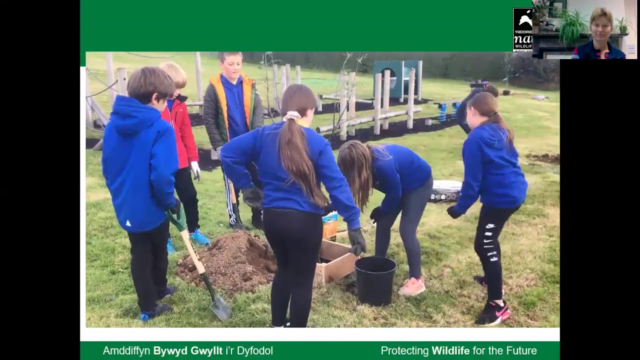 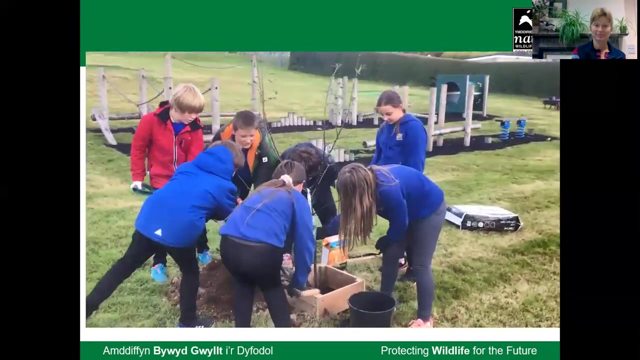 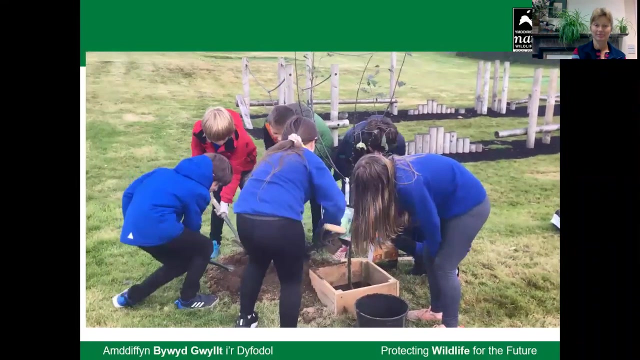 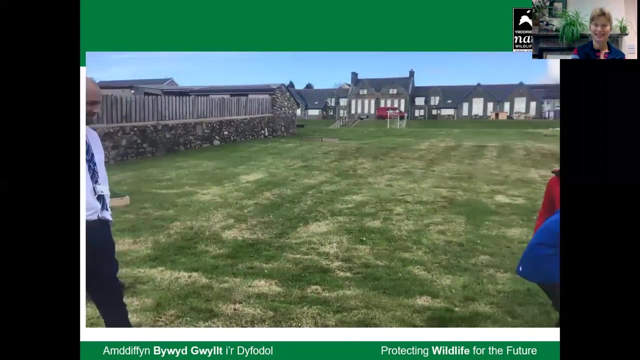 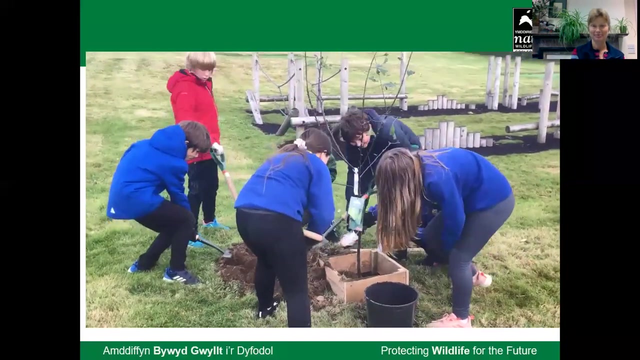 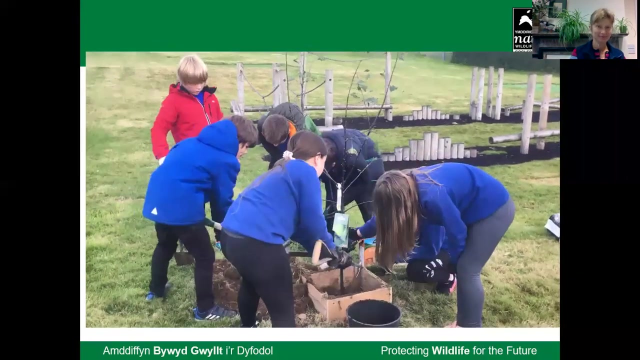 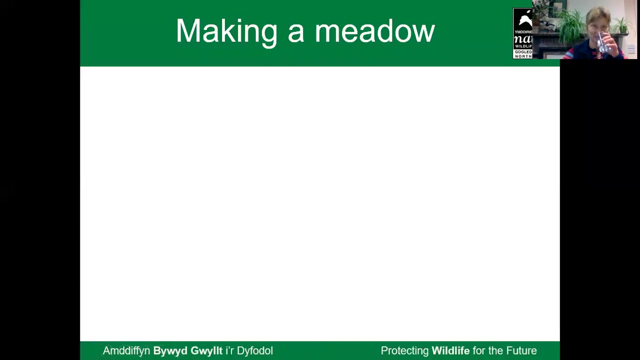 of the pot. here we have a bit of calamity going on. you satisfied headmaster, the system right, so anyway you can see it was good teamwork. I must say they did a very good job at planting that up a tree and it's great to see them working together. 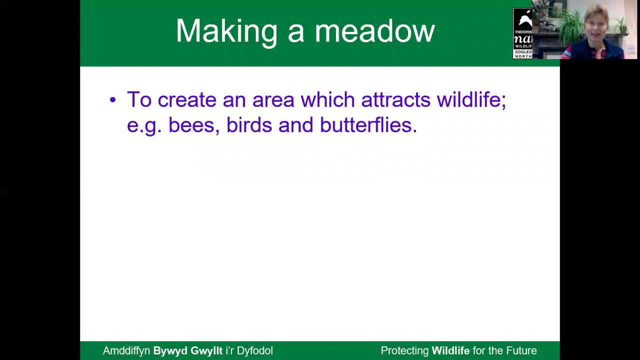 working out how to do it, so making a meadow. meadows are excellent for wildlife, for all our pollinators, and they are increasingly disappearing in our countryside. we lost 98% of our meadows in the Second World War, so if schools can create meadows, that's fantastic and obviously it's a great area I mentioned. 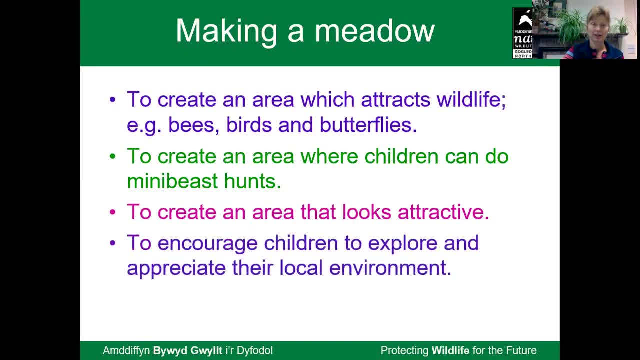 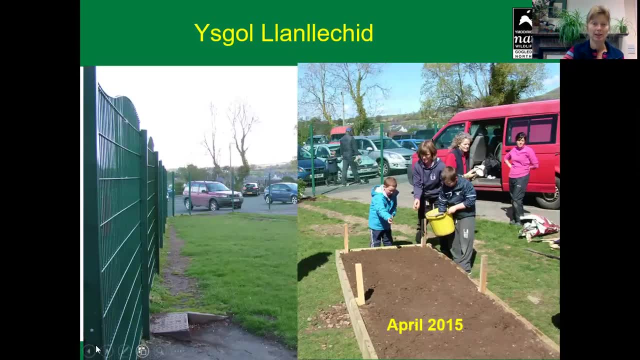 you can do mini bee hunts and look attractive, and I'm just going to show you some examples here in Clarke. here they wanted a meadow but if it's hard to make it from this open bit of ground and we needed them to create an area, so I did a box like a veg box, really raised bed and 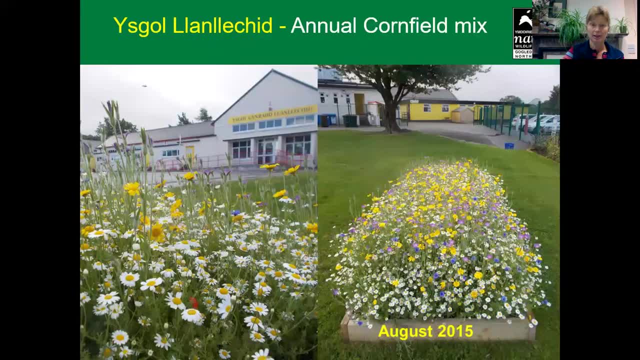 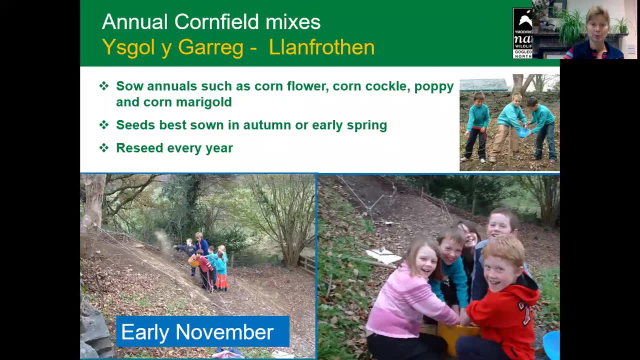 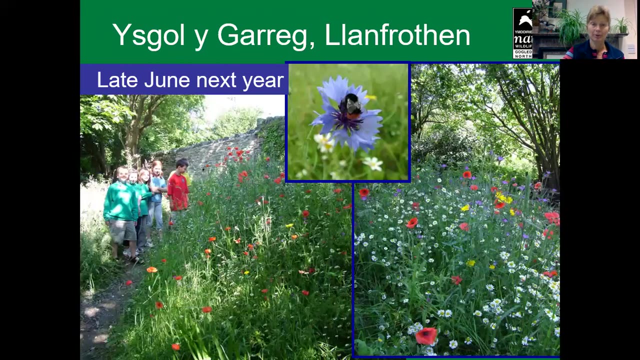 this was a group with the special needs of planted in April, and in the following summer I had a fantastic display of colors. if you plant a little earlier in the autumn, you get the flowers earlier as well, and that's in Llanfrossan. we had lovely cornfield mix. 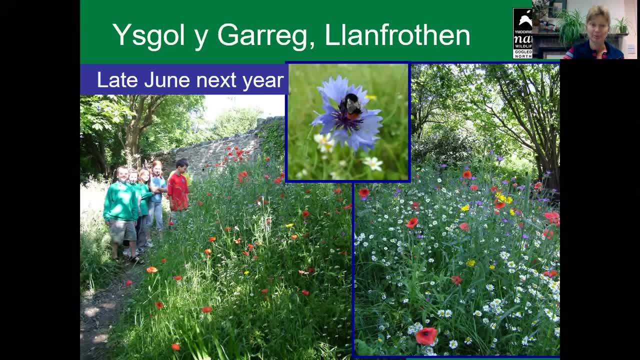 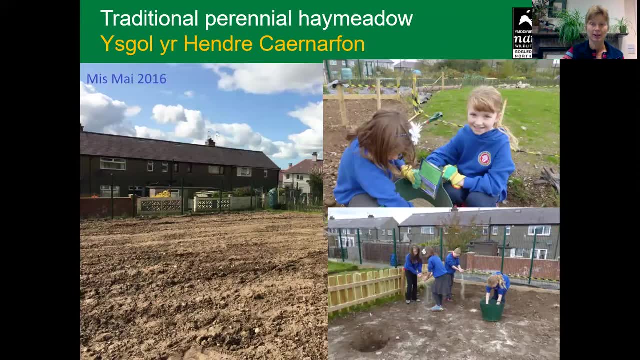 which are good for the pollinators, as you can see there, the red tailed bumblebee Hay meadows, the traditional ones. those are perennials. they come year in, year out, but you have to cut and remove the hay every year and you can see the pupils sowing, and we were also doing a meadow together. 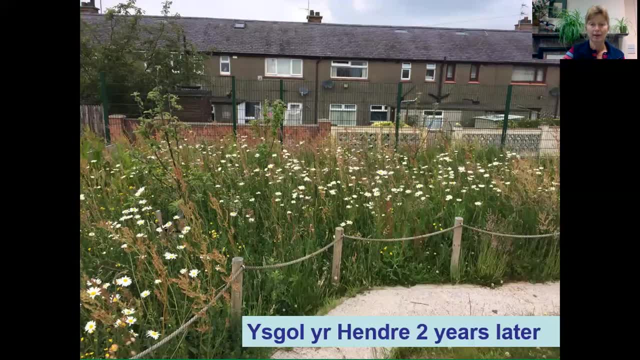 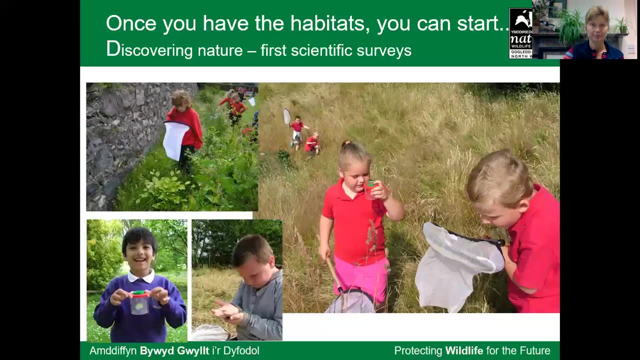 with some apple trees like a little orchard here. I was very happy with that result, but it has to be cut and removed every year at the end of August. Once you've got the habitats, of course, you can start doing your own surveys, scientific surveys, and I yet have to meet a child who doesn't enjoy. 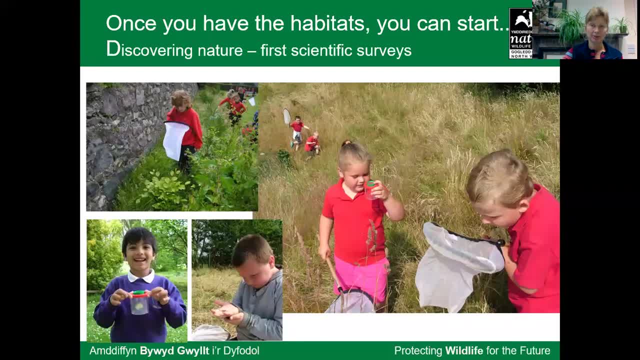 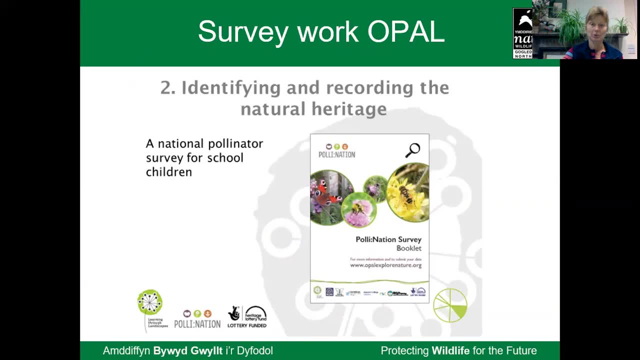 catching a bug and you can record everything and you can make as much of it as you want. There is a very good organisation in Llanfrossan and it's a very good organisation and it's a very good organisation called Opal. they have resources online, all different surveys. this is pollination. 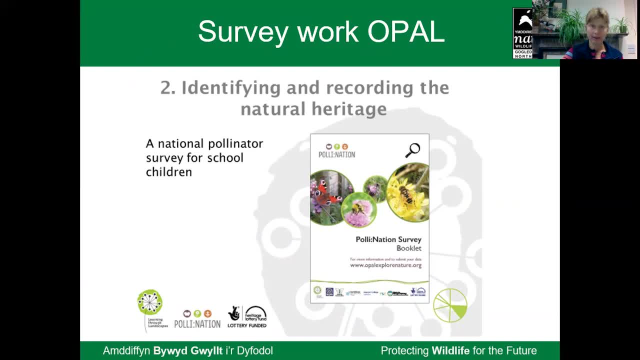 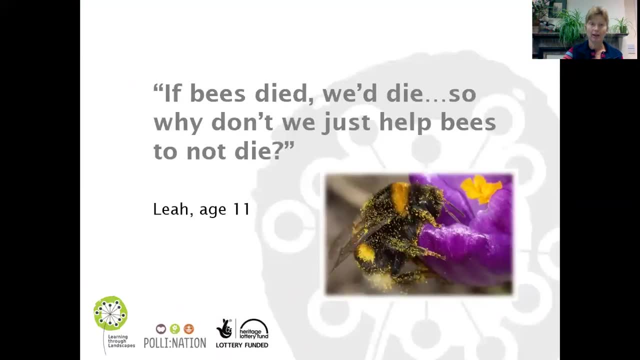 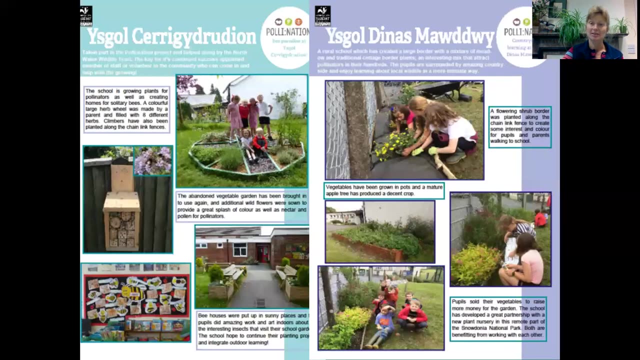 one. there are others: soil surveys, bug hunts on surveys, etc. all available online for you to use. I was involved with this pollination project- and that's quite a poignant quote by Lea- so we got involved in improving school grounds for pollinators. This was actually a project that was 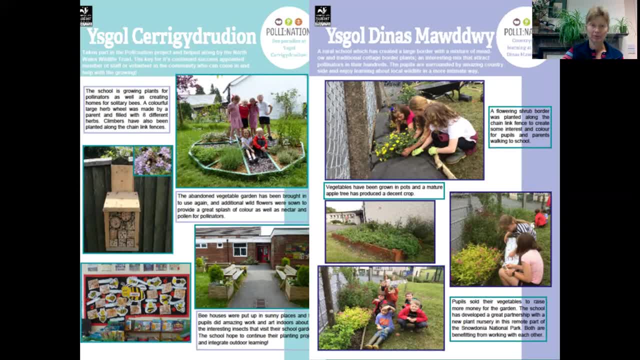 eight schools I worked with in Northwest Wales. I worked with four in the North East and we're doing everything from making nesting boxes for solitary bees to habitats- that's a wheel again- planting along the fences, and then they were learning about bees as part of their school. 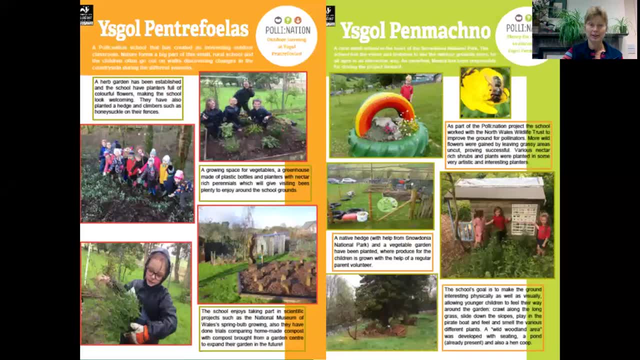 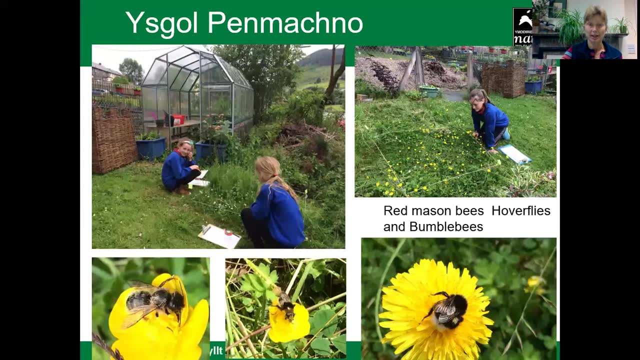 day. Here are some more projects and in Penmachno you can see we were doing recording. it was quite interesting- I was there helping them with the Opal survey- how much we did actually find in this little patch obviously, where you leave the grass to grow and you might get buttercups and 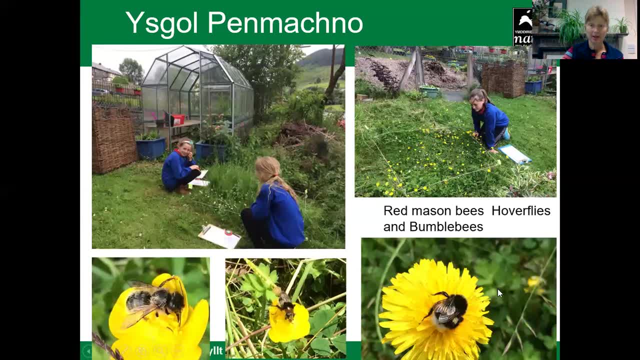 other flowers coming through, you will get the pollinators. And again I must stress, you don't have to be insect expert to do these things. they're very easily described for any amateur. These bits of land- this is in Llanfrossan and Penmachno- are very, very good at conveying knowledge to the birds. 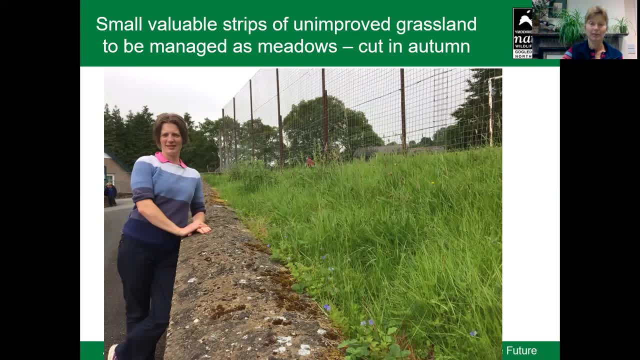 Hymnaskálp en Máfnáw are very, very good teachers and I would say they are very good at grasping the data before they come to the species, are very, very good for wildlife and I was surprised by how many different. 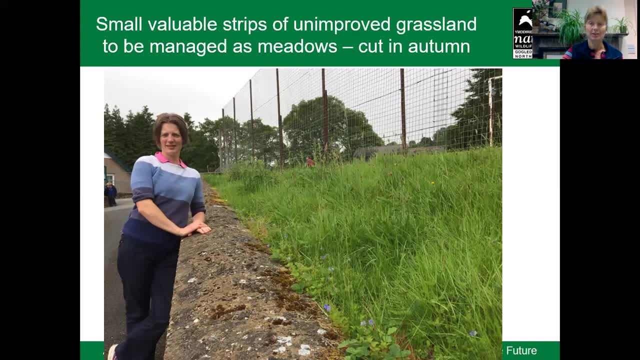 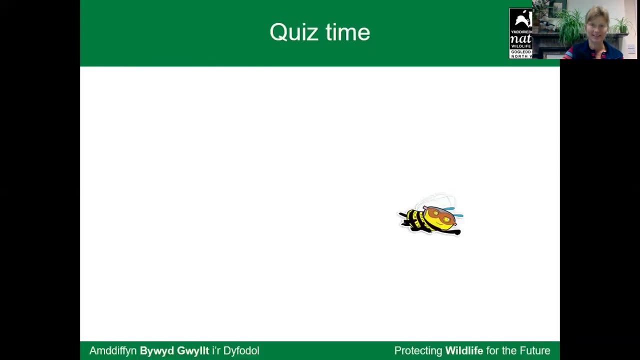 flowers we recorded in just this strip. so some of its schools will have areas that haven't been improved or fertilized, and those are usually much higher in wildflower numbers and then obviously also in pollinators, because that's where they go. right time for a quiz for yourself. get a break from my voice. so. 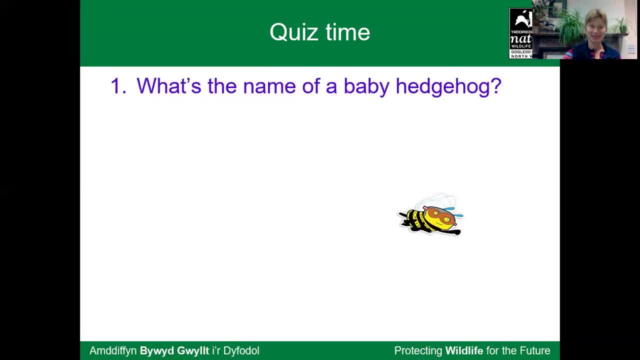 you can do this for yourself and then afterwards you can tell me how many right there you got correct. I've got six questions. what's the name of a baby hedgehog? why do our trees drop their leaves in winter? all things you can ask your pupils. which continent do our potatoes come from? our beetles, part a. 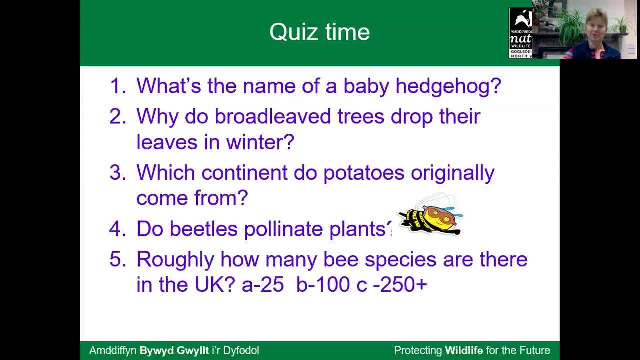 pollinator and how many bees species are in the UK. a lot of these children are like sponges. you know that. so now, when you're young, it's brilliant time to learn, and they've got very good memory. so certainly this- the plants I learned when I was younger. all that stays much better, even as you. 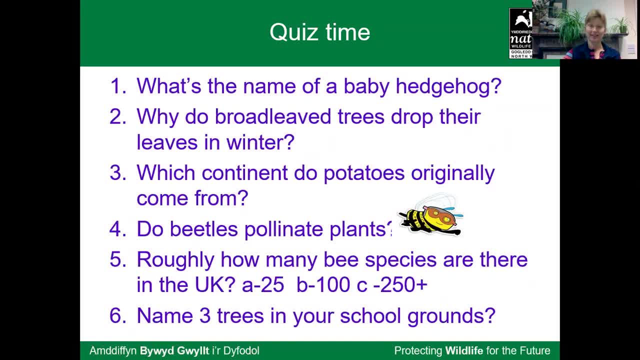 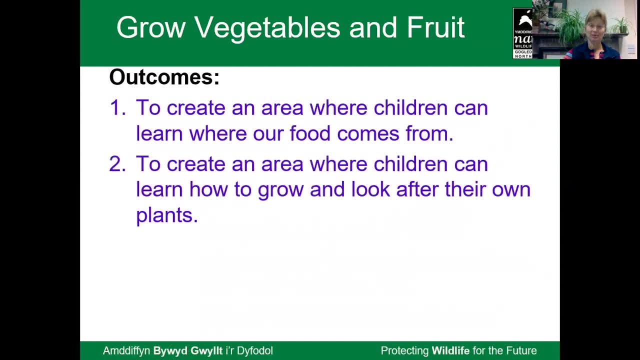 grow old. so, okay, we'll go to the answers later. coming on to vegetables, obviously, where the food comes from, how we grow it, how we look after it and then harvesting it, and many pupils have eaten food from the garden they'd never eat before. certainly somebody came out to. 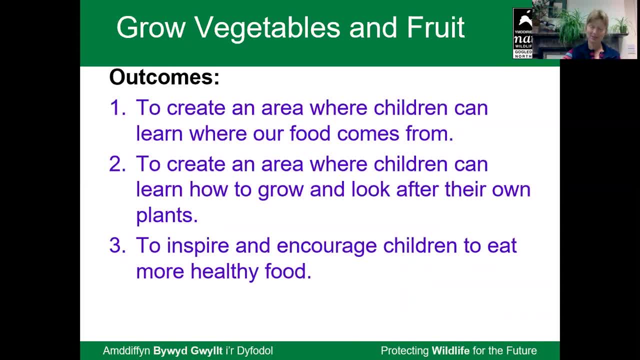 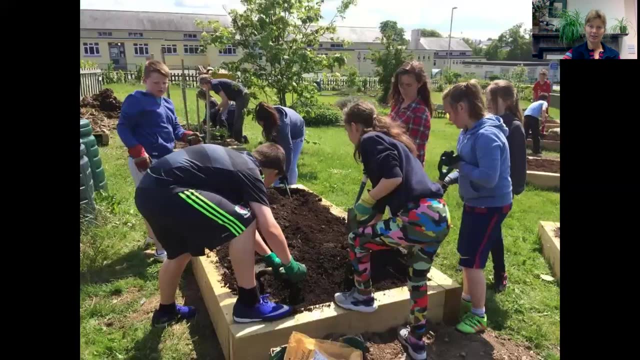 that. who are we doing cabbage for the first time, and that is once. that is inspiration. once you grow in it, you do want to try it, and it's also a reason to go outside because the veg garden needs care throughout the growing season. here the kids are getting the hands dirty in Carnarvon. I really appreciate the kids. 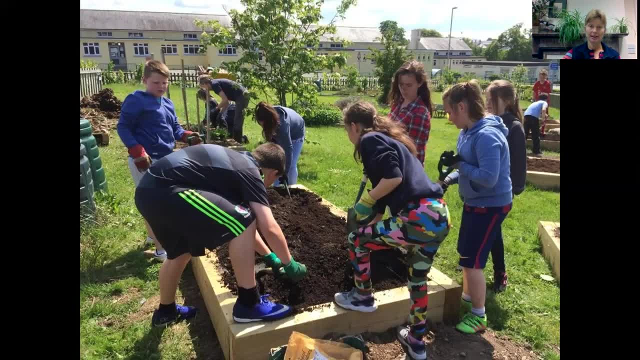 getting their hands dirty in Carnarvon. I really appreciate the kids getting their hands dirty in Carnarvon. I really important to do the digging and digging, as Monty Don will say, it's very good for your mental health, it's good to release any stresses and for pupils who maybe 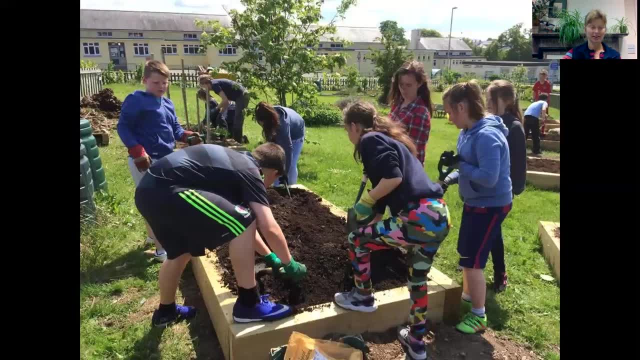 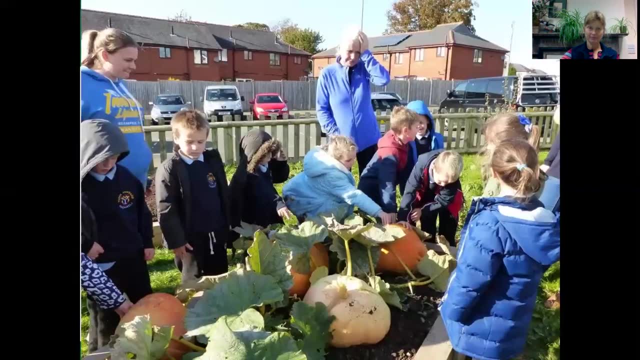 are suffering from different stress related problems. they can get a good release by going aside and digging and chatting. little kids got involved with harvesting the pumpkins. too heavy to carry, they're absolute monsters. I must say I'm very impressed with their pumpkins this year. and here's a group of boys who have harvested potatoes sweet. 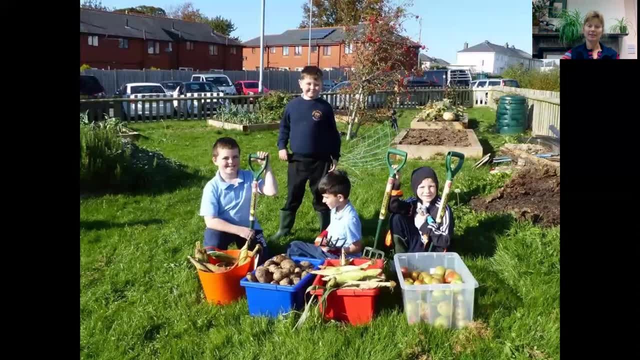 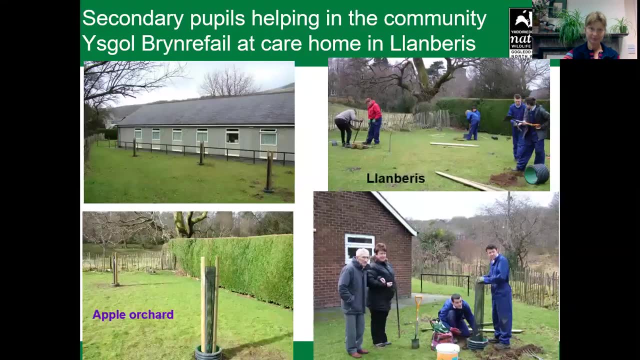 corn and some apples there, and this photo was actually in the local paper and I think it's that's important to do. share what you do with a community. we don't only need to do the work at schools to take in a school green. we don't only need to do the work at schools to take in a school green. 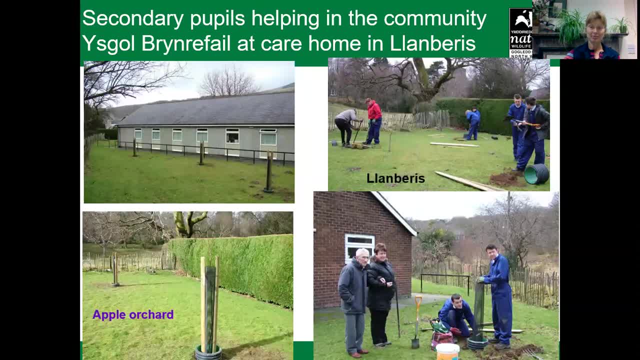 with us. I would like to stress that I hope that this video has been useful and we will see you soon in the next video. today, now, we should know what to do with the Christmas tree. ok, people, today I write in writing, and it's in clam berries, and the sheep roam freely. of course, apples are great, so with your apples. 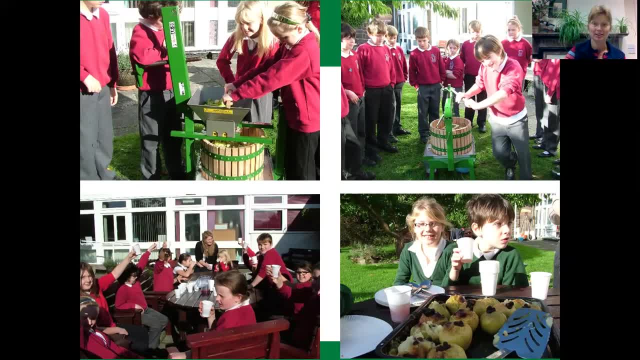 from your garden. i planted an orchard. yesterday- actually i was in askalpadapan- and you won't have this many apples next year, but in years to come you can make stuffed apples, and here we are making apple juice, and this was on the conway food festival where a number of schools got involved. 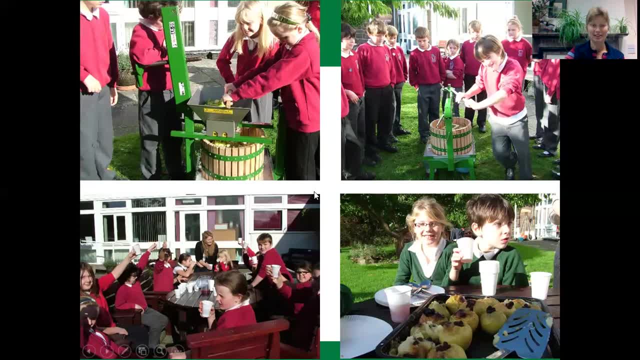 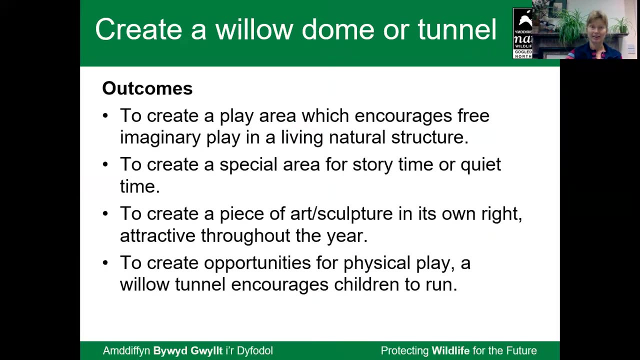 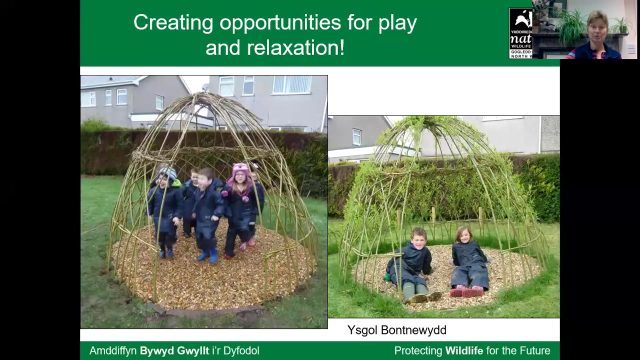 with making juice with me. the children were so excited. it is brilliant. i'm making some cider at home with them, intellectually, and it's really fun pressing it and the juices taste so much nicer than shop bought juice willow domes. they are great for play relaxation, but they do 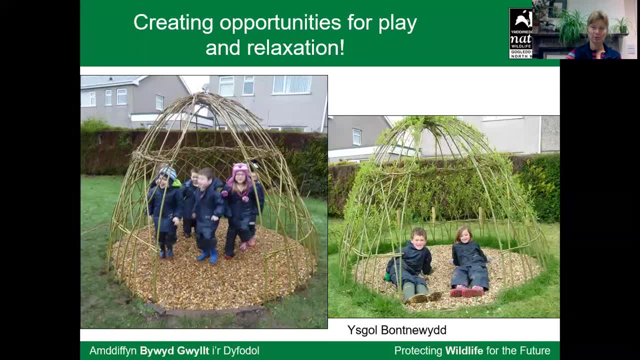 definitely need maintenance and some schools have been a little bit poor at that. So every year they need cutting back or weaving in. So if you do a Willow Dome, do think ahead that they are a source of work in years to come. But obviously it's only work and if the kids enjoy it, that's great. 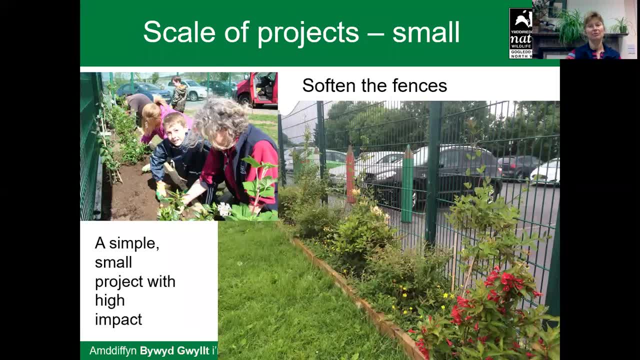 So going to talk about more different size of projects I mentioned. they can be small and small, as here we are planting a border along a fence and my colleague calls it de-fortressing the schools, all the non-climbable fences that you have. 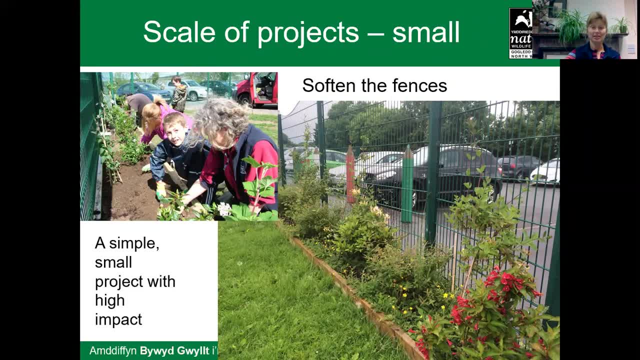 around the schools. They are a bit harsh, and so the benefit here is for the parents- they get a nicer view while they're waiting to pick up the children- and obviously for the wildlife. they have got plenty of nectar and got honeysuckle and other shrubs growing along the fence. 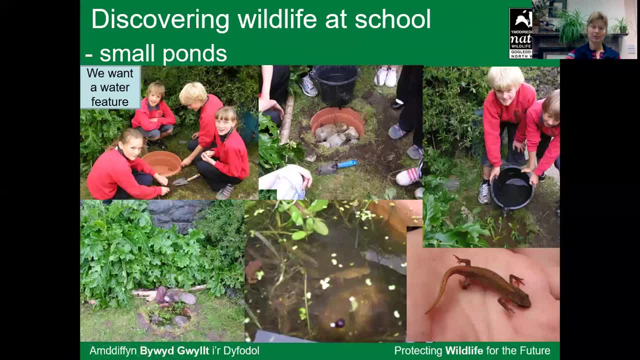 Many schools don't want ponds, for obvious reasons. but you can make a mini pond like this one, Only a small flower pot and or a washing up bowl, and I was absolutely amazed when they said the big pond had been finally in use in this little pond. So this particular 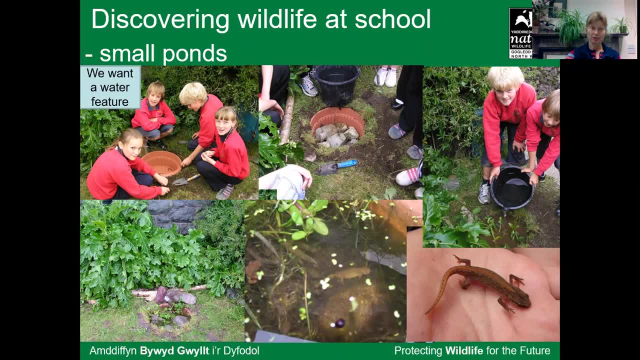 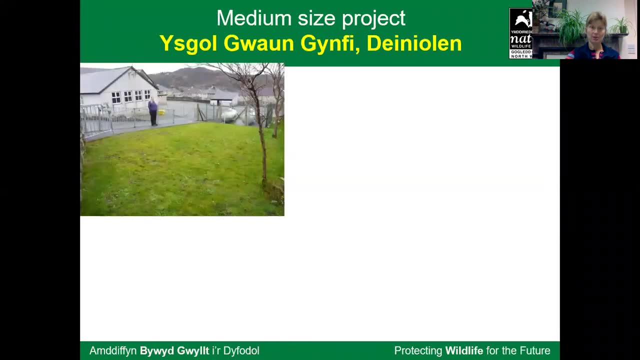 part of the garden was in an area where the children can't go anywhere with their teachers, So it's a good place to put a mini pond, Medium-sized. this is classic piece of green grass that wasn't used up in Daniellen and the eco teacher was asking me: how can we develop it And together. 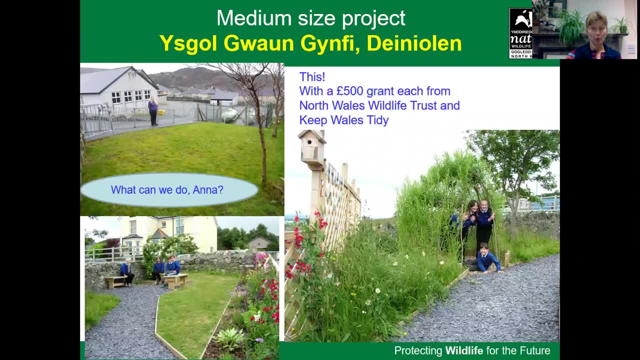 with parent and mentor Farhwen. it's a learning center for people with learning disabilities. They came and put up the trellises, We planted a meadow, Made a willow dome and then this flower border And it's- yeah, it's great to hear afterwards the teacher was saying so much easier to teach. 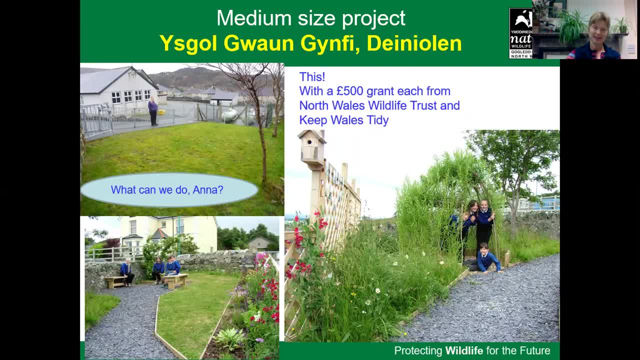 the children about flowers and pollination, as we can go outside and children can take the flowers apart and have a proper look how it all works. So having it for real life makes it that much easier for the children to understand and for the teachers to teach. 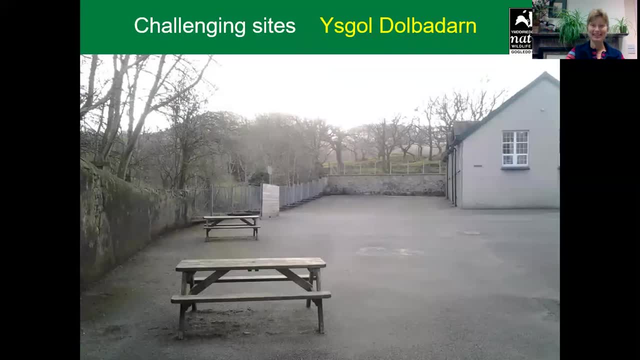 One or two challenging sites. I was a bit daunted when I came here, thought how can we develop this area? It's in Llanberis and the school has one of the most stunning views of Snowdon, just up to the left there, but the yard leaves a bit to be desired. 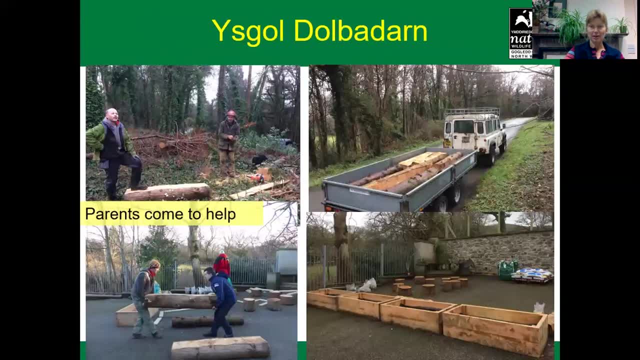 So we got they were part of the pollination project and we had a meeting and there were parents who were willing to come and help. I begged some trees from National Trust Henry Castle site. always ask others for materials and you might get it for free. 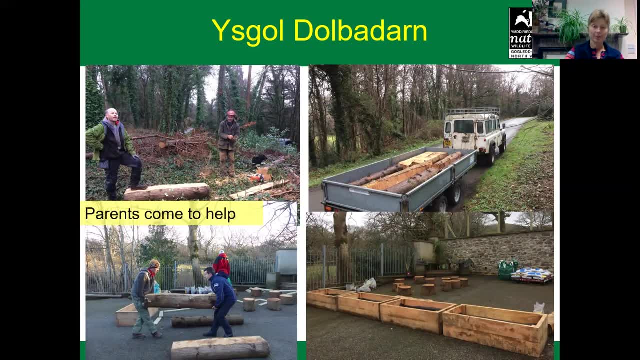 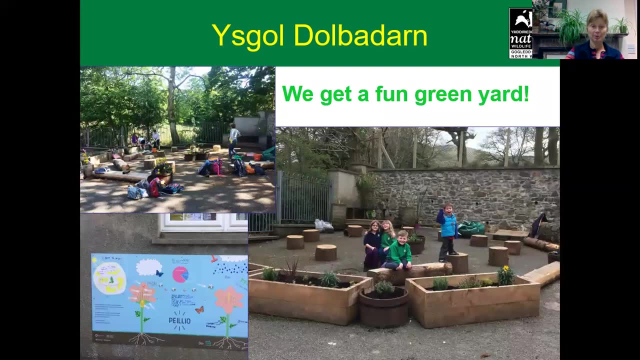 We got all these logs for free, and then a parent made these lovely wooden boxes and the children planted them up. So in time we're hoping to create a green screen and, not surprisingly, the teacher was telling me that this is where a lot of children go to play now, in during playtime. 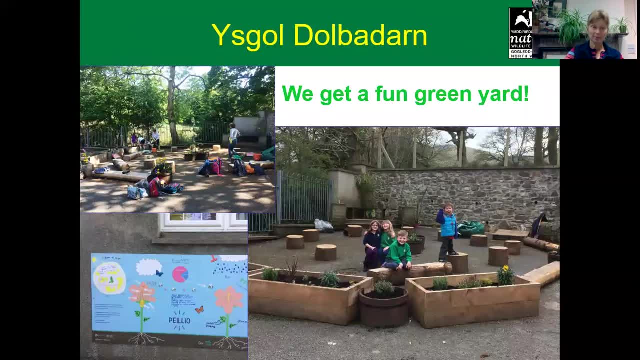 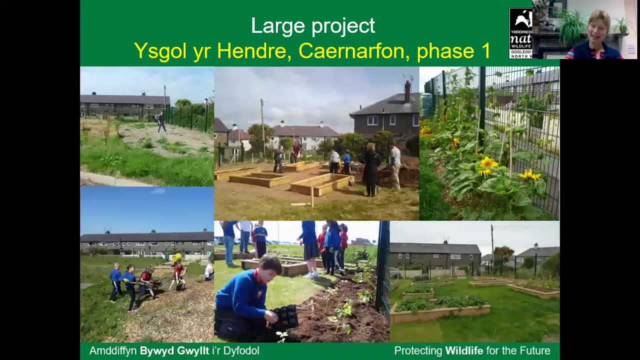 It's a little bit more inviting, I would say, And on the wall they made a big artwork about peclio and the pollination process and projects processes that we're always looking for. Okay, so Doon Shadad can brag- held it. 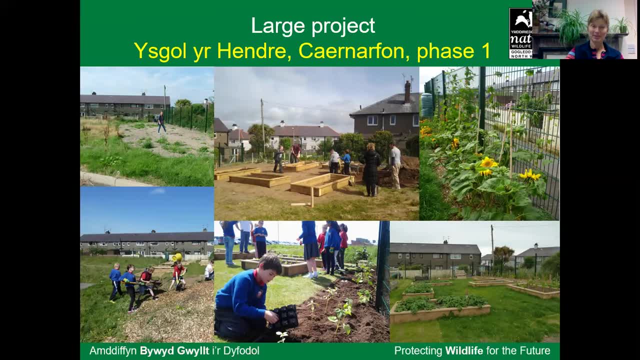 Doon Wedi Dusky can brag. I'm doing Shadad over the plants, So I am Swedish. I have learned Welsh, so I do speak Welsh, and a mixture of everything when I'm out with school children, but they love it and they can teach me as well. 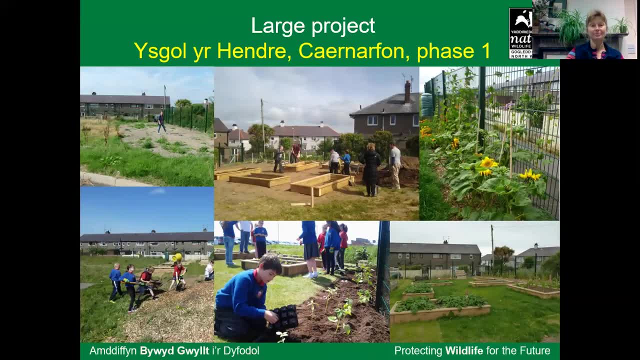 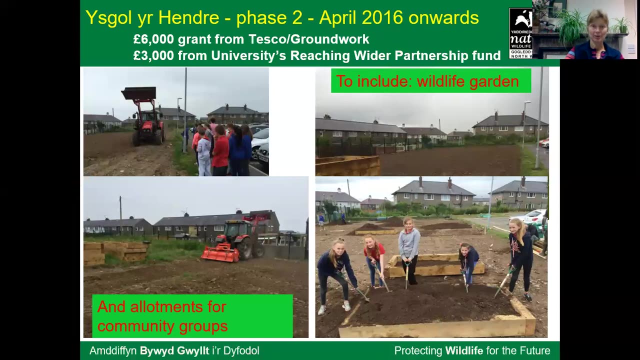 This is a large project. as you can see, in Caernarfon We started from scratch nothing. The previous headmaster thought the whole ground there bordering the estate could be developed for allotments and wildlife gardens. I helped them, actually with a grant, and we got £6,000 from Tesco plastic bags and we 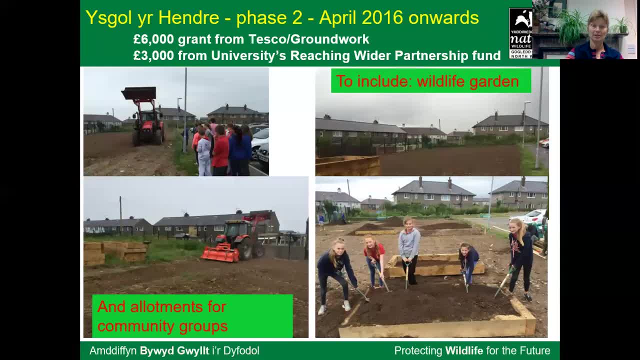 got some money which paid for my time, because I also need to find funding to pay for my time when I'm helping school. So first time I did school gardening with a tractor, but we had to get it in for the site prep. And here the girls. they've been moving about a ton of soil. 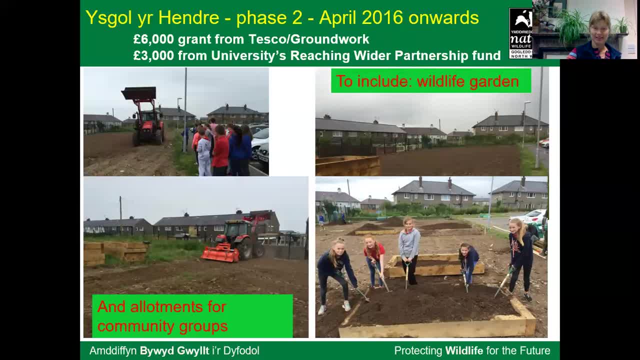 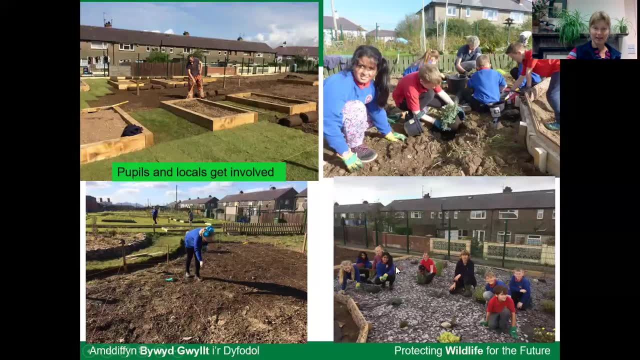 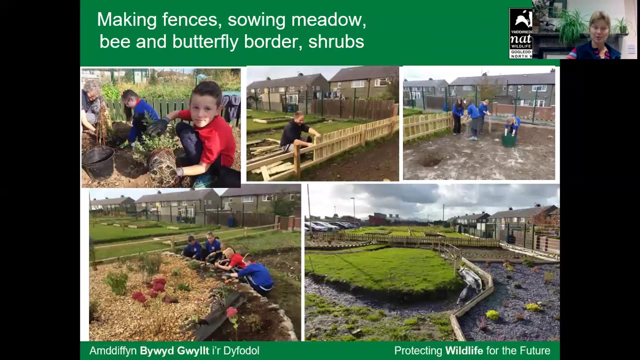 We had a little competition. Girls were faster than the boys and they were filling up all these beds. But no great stuff- A lot of work, But It's the process that's important And I certainly had a lot of good feedback from the teachers. 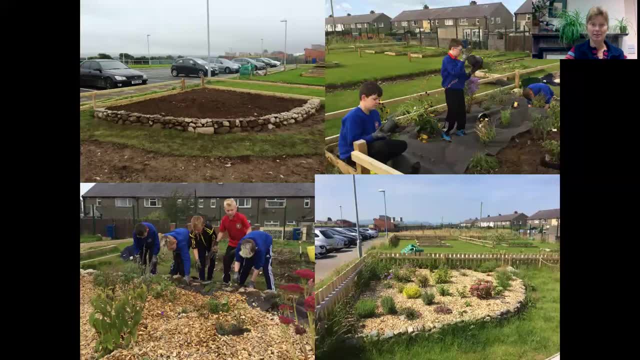 And certainly some days I would come in there. I could sense that the atmosphere was tense in the classroom. I took a few pupils out and they got digging, raking or whatever we were doing, And the stress seemed to evaporate and we were having a good time. 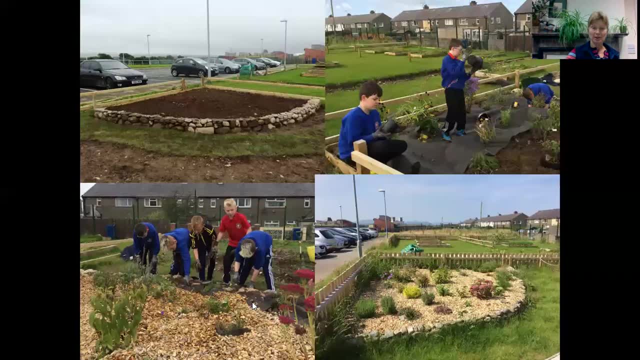 And I just want to show here the boys in this picture in the bottom left. they came out in their playtime to finish off the project And I found that with lots of projects the kids are so keen they actually come out and stay in playtime and lunchtime to do the work. 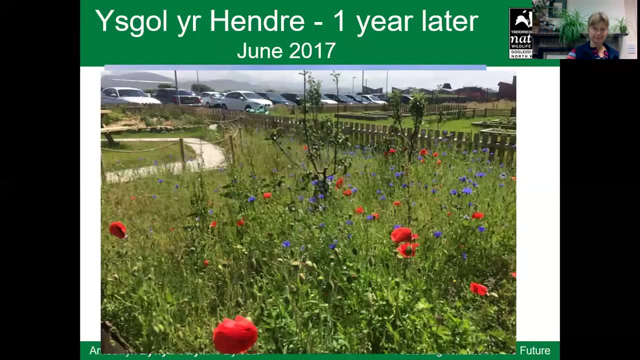 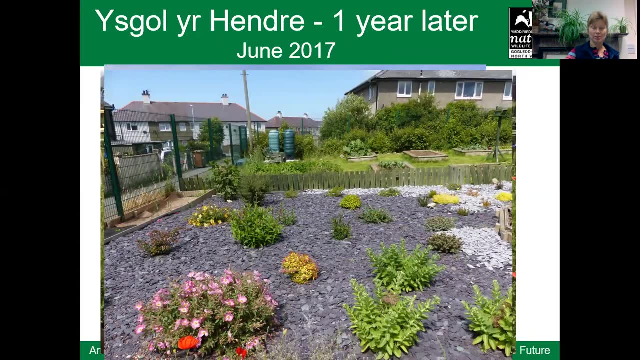 So just quickly show you what we did and how this site has been transformed. That's a shrub border which looks a bit empty, but now it's a lot fuller. So do plant things with a good far apart so that the shrubs don't fall off. 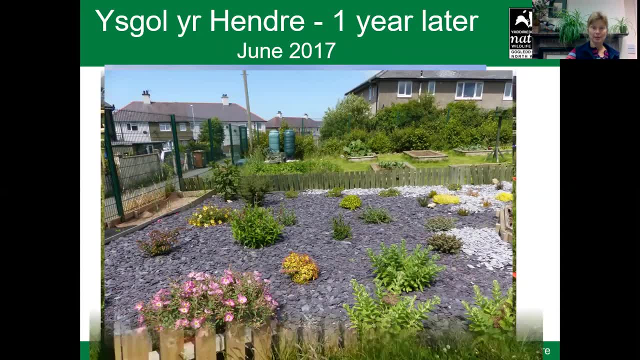 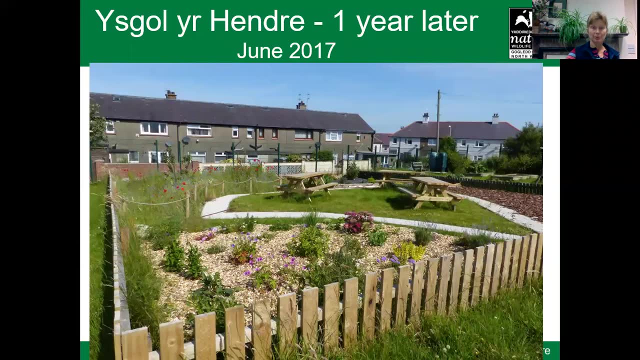 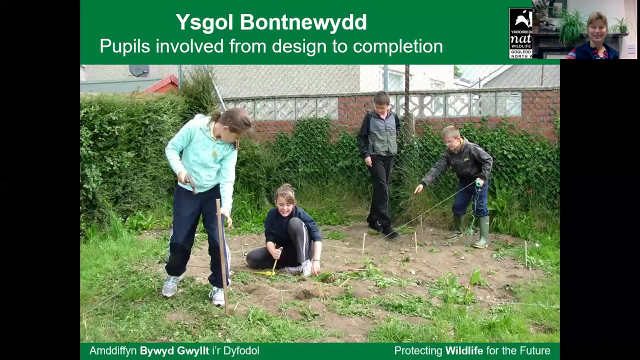 Some people were a bit negative and they said that this area wouldn't be left alone, It would be vandalized. But we haven't suffered very much at all there. Now I'm just going to show you another project which we've been there before. 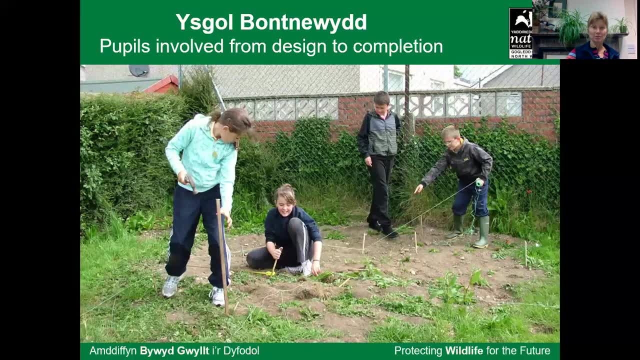 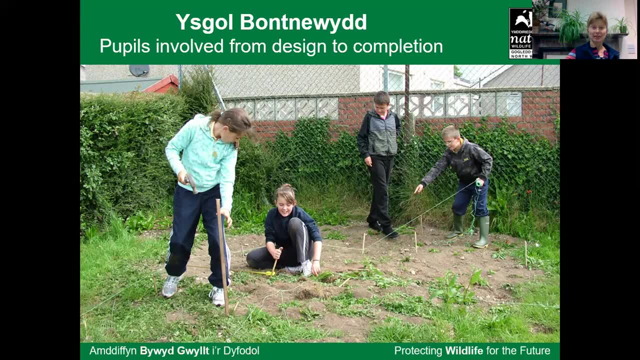 I found the girl there on the left hand side of the picture. She was kind of most on it with a practical marking. So I made her the project manager for the morning And she was trying to organize the rest. And when I came into the classroom afterwards and we talked what we'd done and they came 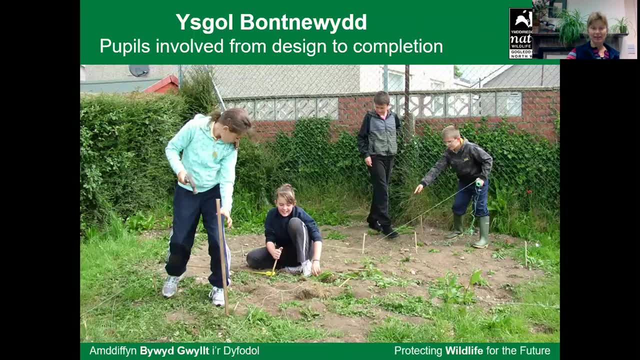 out to look. it was lovely because the teachers told me that she's very dyslexic and she doesn't particularly enjoy school And although this day she was definitely shining and she had taken the lead And that was great to see. So I'm going to just show you a few photos that have developed. 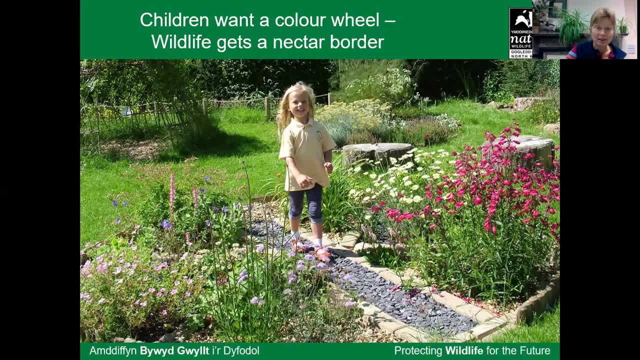 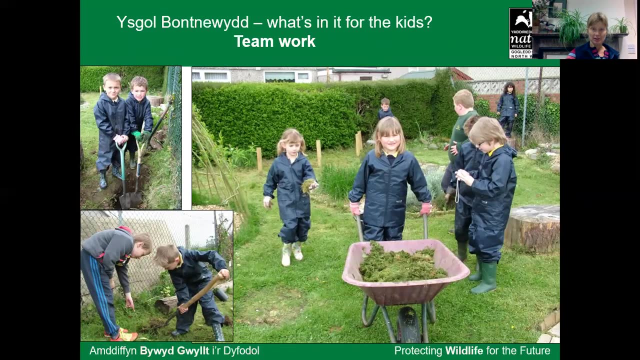 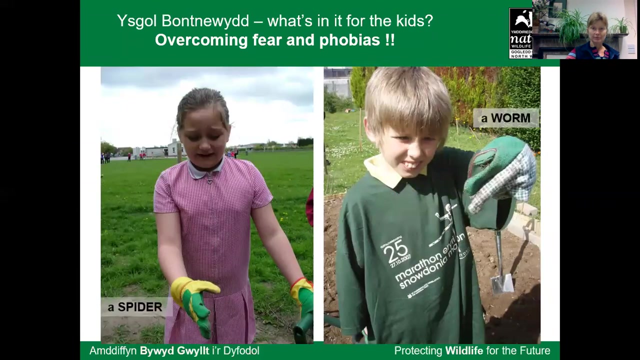 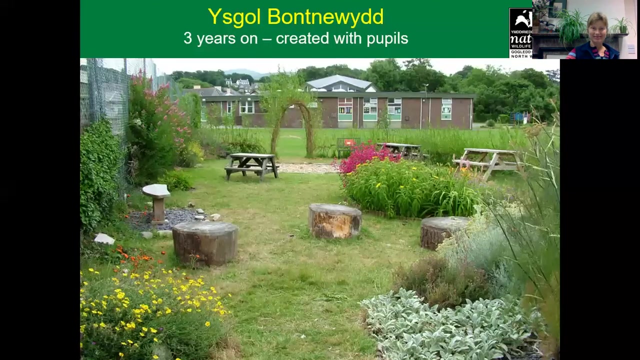 I won't do so much talking. You can have a look This particular wheel. We've done the herb wheel. You saw that, And now then they wanted a color wheel. So we did each segments with different color plants. I just let you have a little look how this is developed. 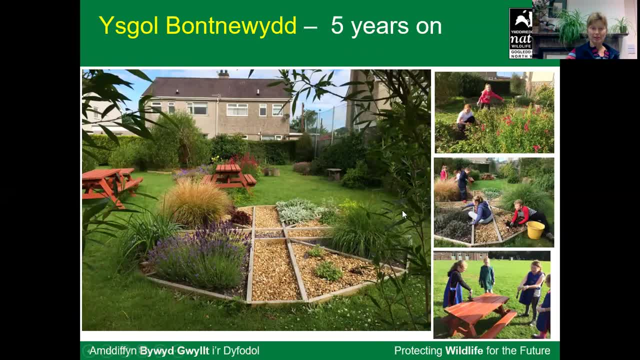 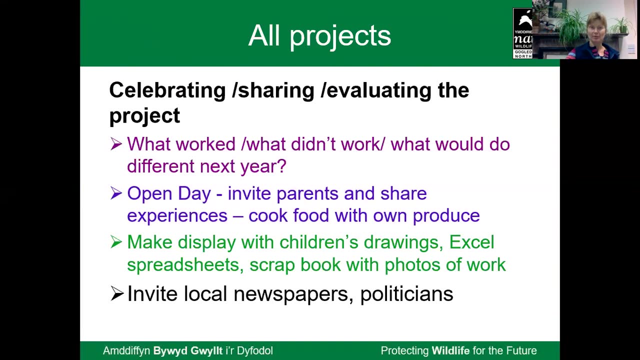 That's a sensory garden in the front. I went back there the other day to do a bit of maintenance. It's going well And that's quite a nice thing to do, To add to any school garden: a sensory garden. As with everything- and I know you do it already- it's important to celebrate, evaluate your 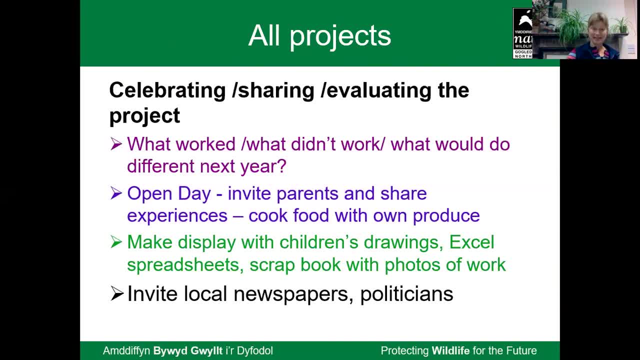 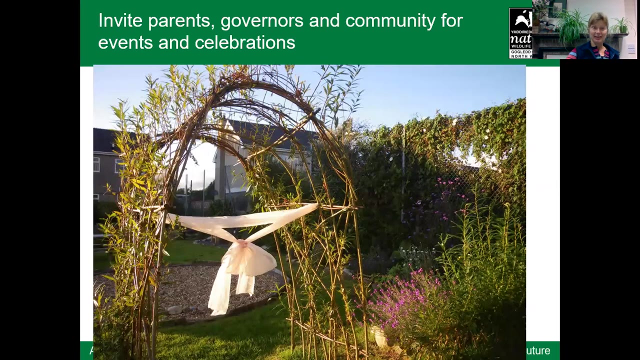 work, Tell, tell people, tell them, invite the newspapers and politicians, And it's surprising how much you might get back from the community. Some schools get a lot more involvement from communities than others, And here we had an open day, opening the garden evening, which was really lovely. 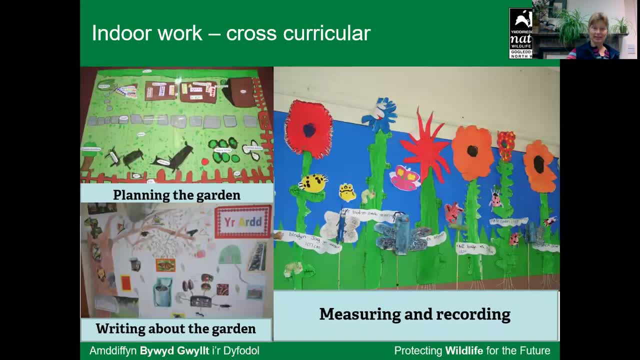 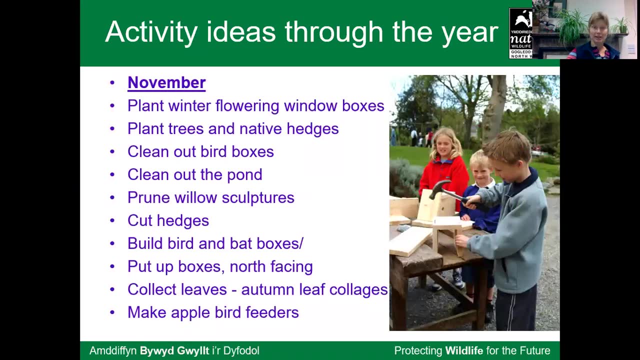 Obviously, all pre-COVID. The gardening work doesn't stop outside. You can get a lot of work inside. What I can give you as well is these activity sheets- different things to do throughout the year, And the Wildlife Trust have a lot of information. 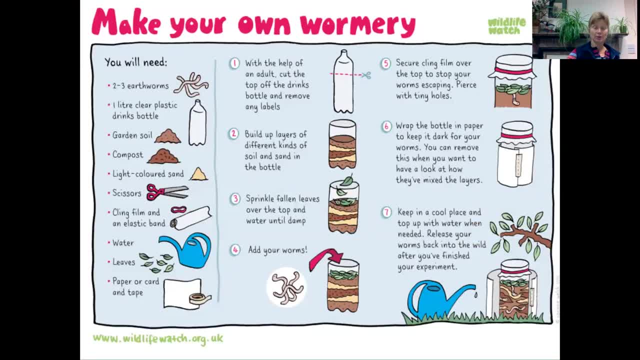 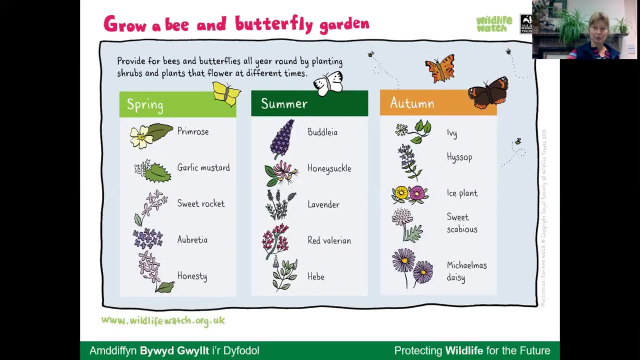 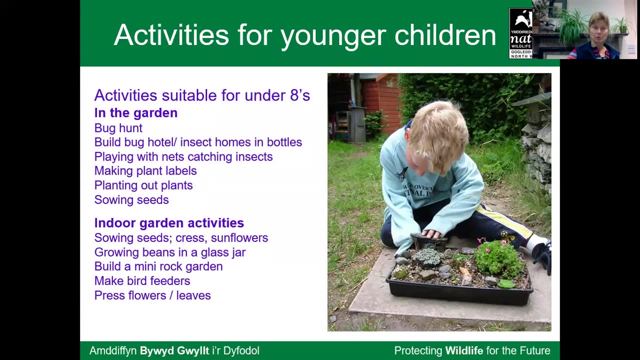 They have a lot of information. The Wildlife Trust have our own ready-made activity sheets And I will mention that later. You can access a lot of our resources if you become a school member. Again, it's not only for the junior schools, but pre-school. 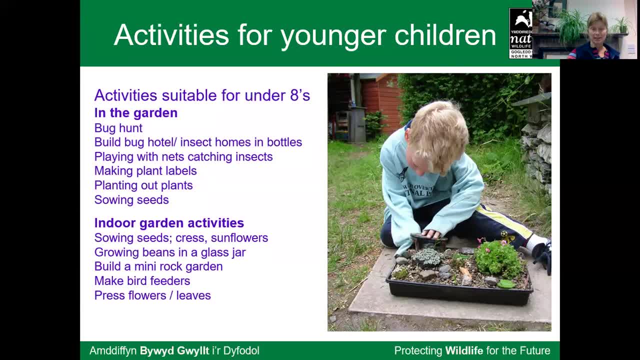 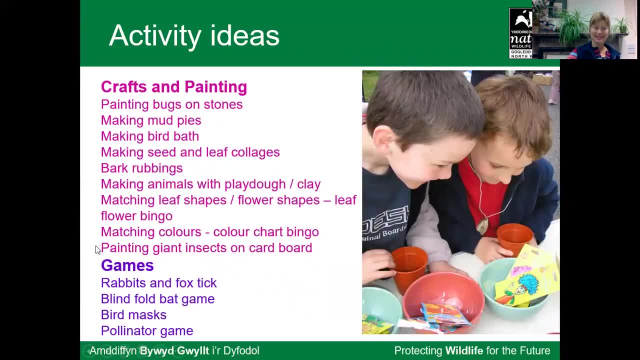 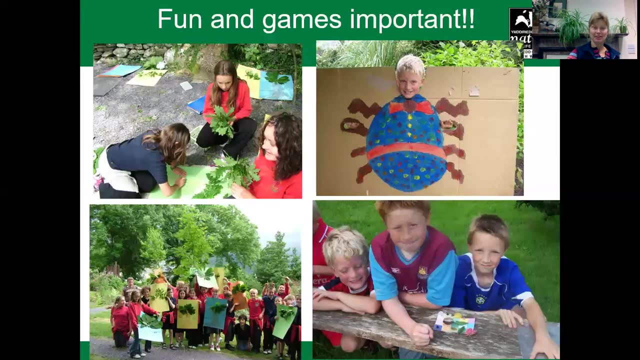 There's a lot to do And I would say for under eights, any of these activities could be done for a range of ages. I'm not going to go through them one by one, But just to give you some idea. Important to have a bit of fun. 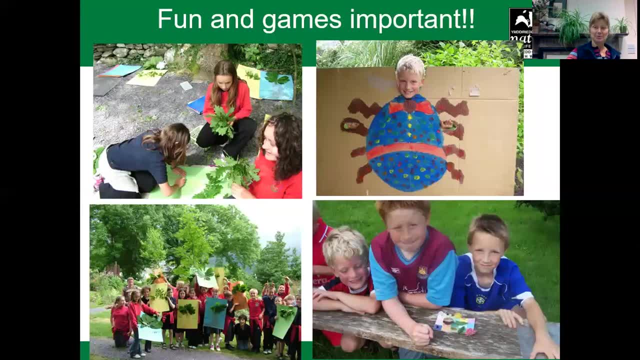 And when you go out there, include games, because I found that with my own children They go out: oh, we were outside, We didn't do any work today, But they learn so much. So as educators, we can teach them without them realizing that they are learning. 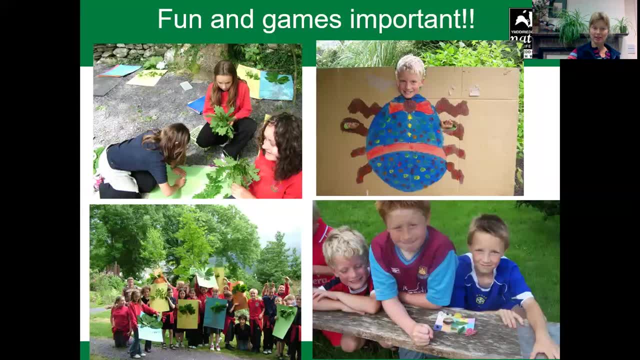 And I suppose that's the best way: Just absorbing. Looking at the shapes, Oh, I think we were doing tree collages here, So we collected leaves And then we made an oak tree or an ash tree, a chestnut tree. 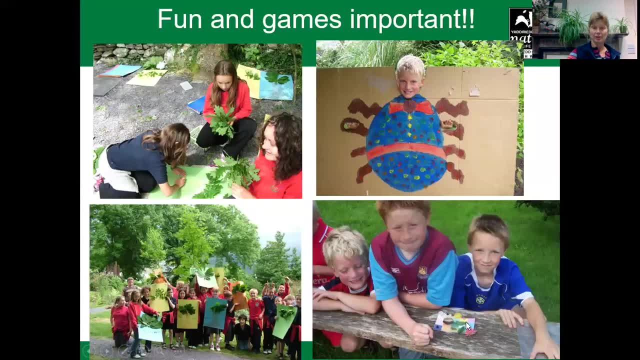 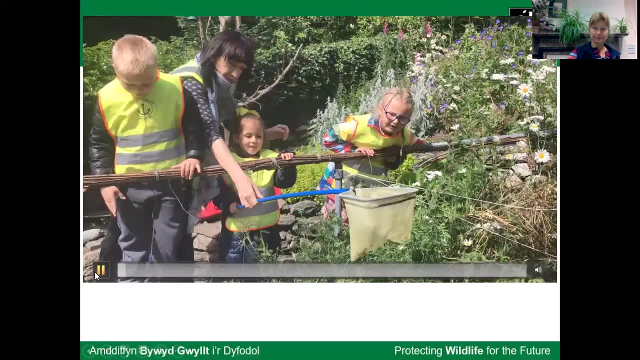 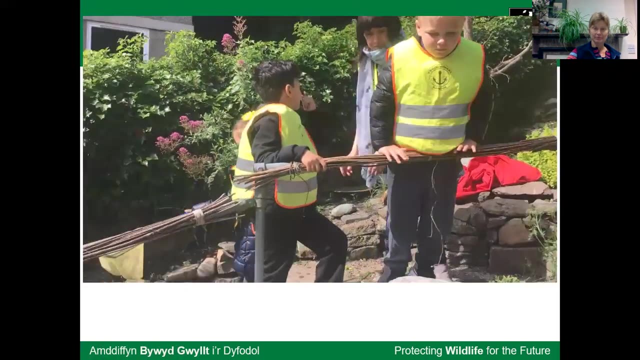 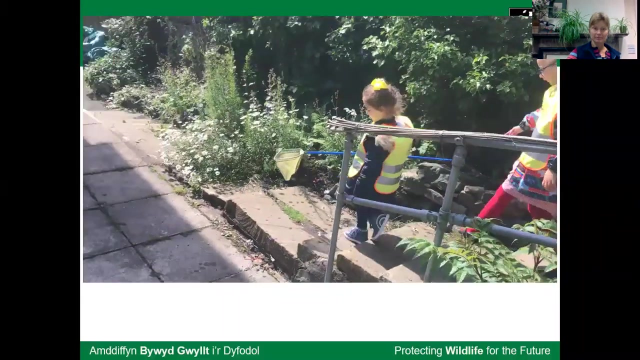 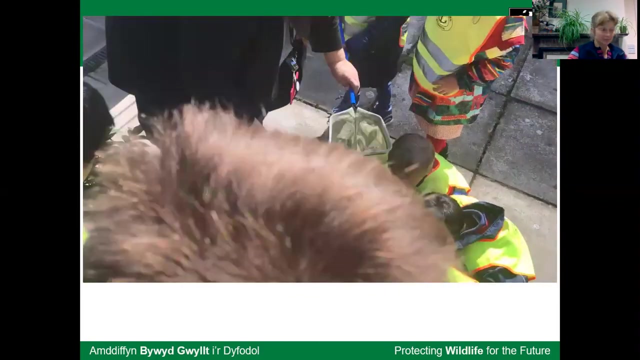 And down here they're doing a color collage. So yeah, Have a bit of fun when you are outside. I'm just going to finish with a little. That is, I don't know So, our teachers. I don't know if you have any questions or questions for John. 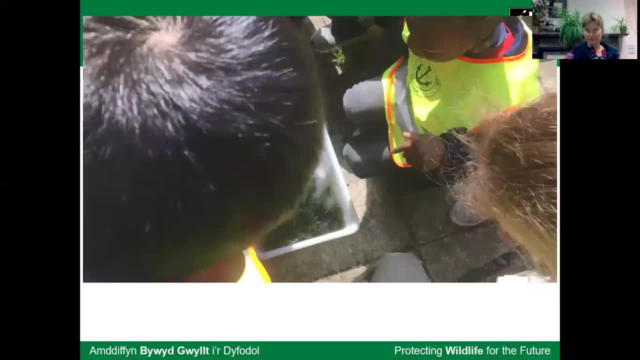 I don't know What. I don't feel it. Ask the child Question. I was at theổ. You're doing a lot of homework, you know. so I was just thinking that's the basics. That's a lot of homework. 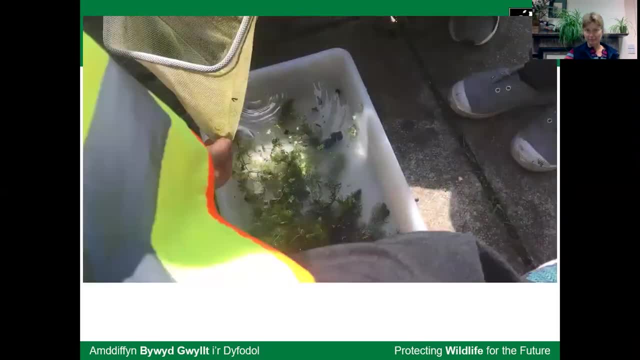 You're supposed to start with the basics. I don't know. Would you mind having a bit of a walk with a little extra time? I know this is a lot of work, But sometimes we're going to have a really boring conversation And then we're going to have a little break. 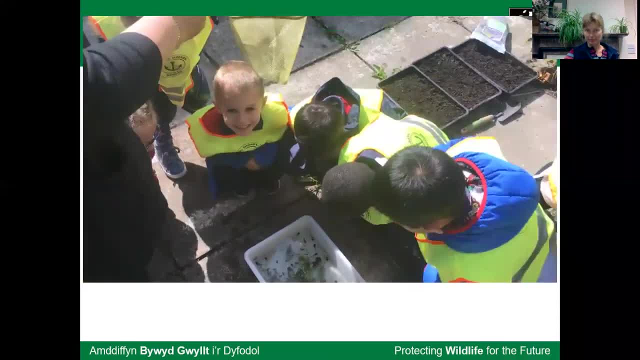 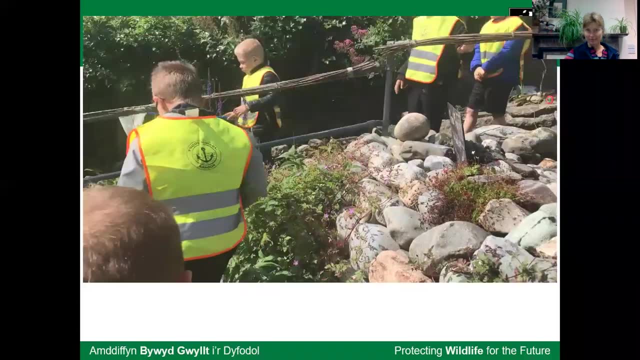 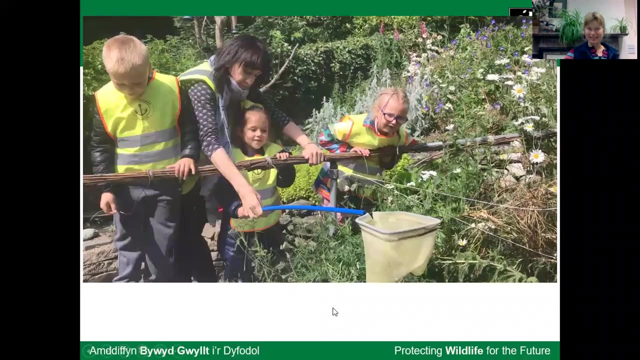 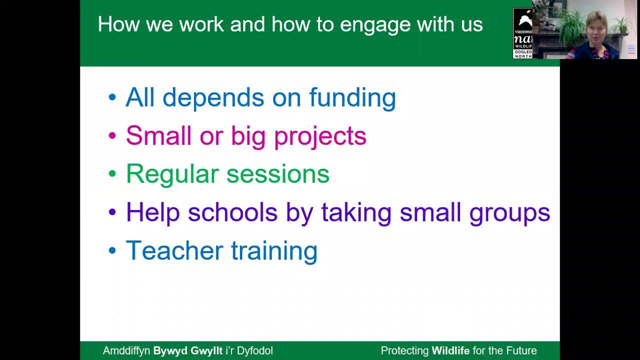 I don't want to do that, But I think we're going to add a little extra time. That was from our garden at our offices here in Bangor. I hope you could hear or get the excitement from them doing a little bit of pond dipping here. 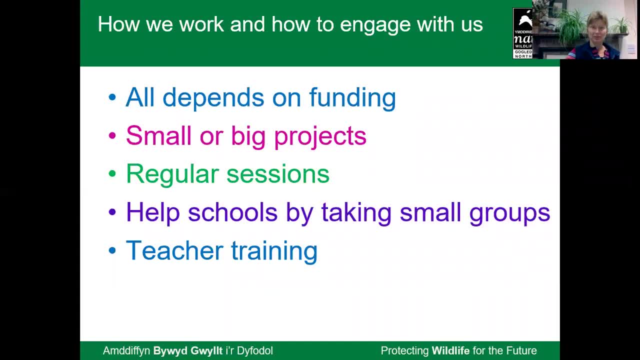 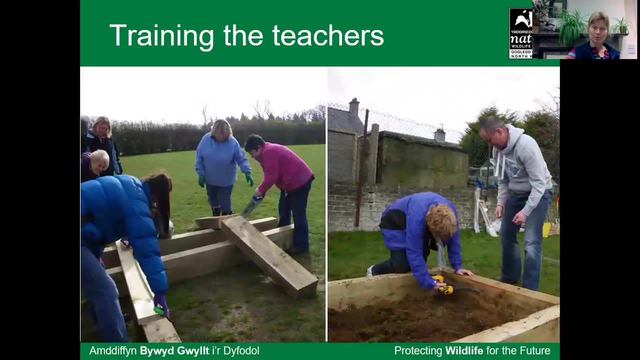 And how we can work with you. it all depends on the funding. My work is never the same from year to year, And if you find funding and can pay in for our time, that's the easiest and the best. Or alternatively, occasionally we have funding to offer, So I do also offer. 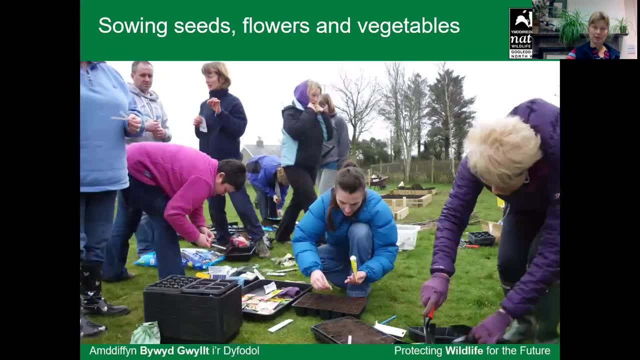 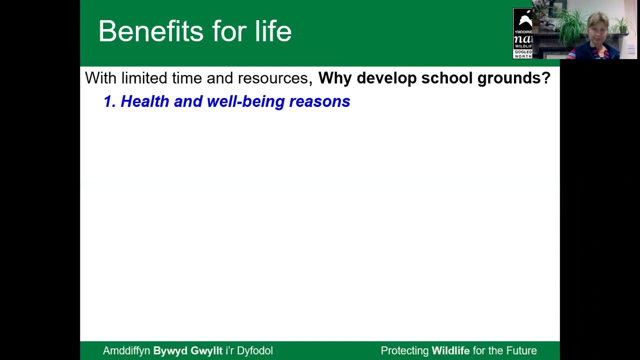 teacher training. less of that in the last few years, but there will be more coming And I just want to say thank you very much to all of you who have been with us today. Let's do a quick recap. So why? On everything I've been going through, the health and well-being 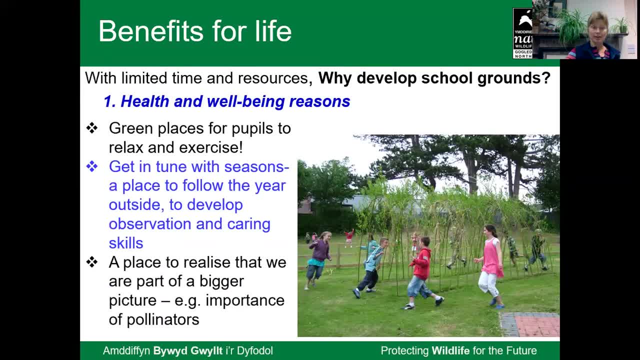 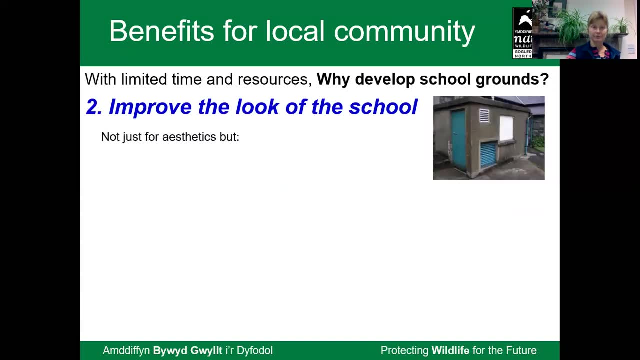 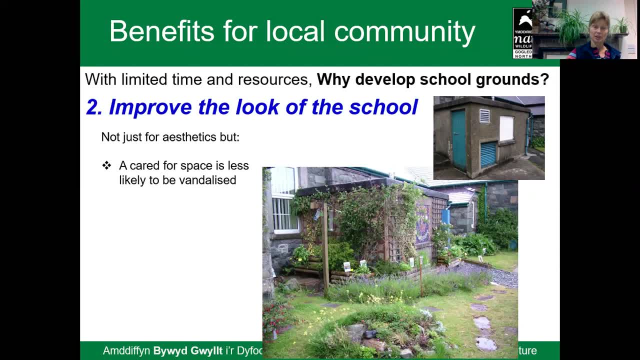 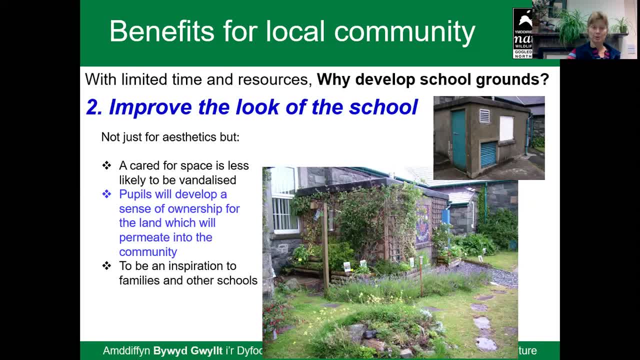 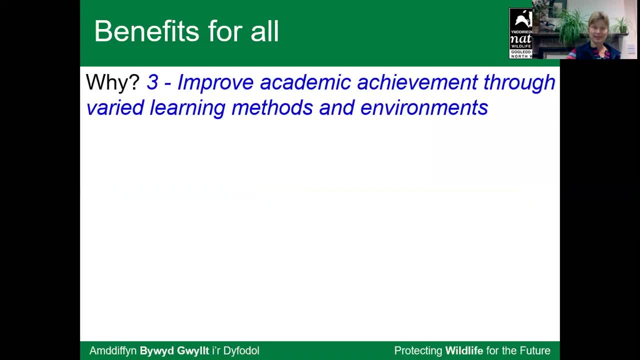 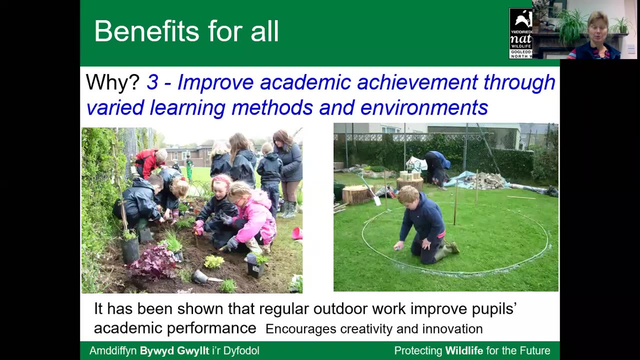 Again, as I said to you, the health and well being is the greatest. It's the thing that is most important, And I think the whole point of this is that in the early days that I was involved in it, there's been a number of studies showing that schools that do do regular outdoor work it also 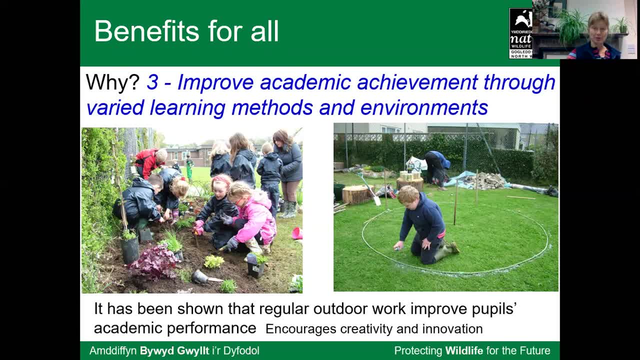 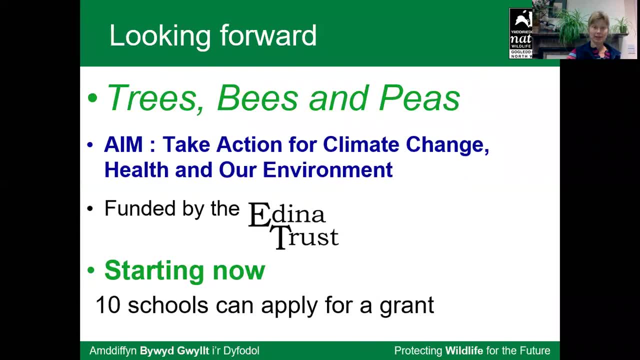 improve the pupils academic performance indoors. I suppose a lot of what I've shown might hint to that creativity and innovation. so for myself, I just got some money free for a project- trees, piece and piece- and I will soon be launching that and ten schools will be able to benefit. 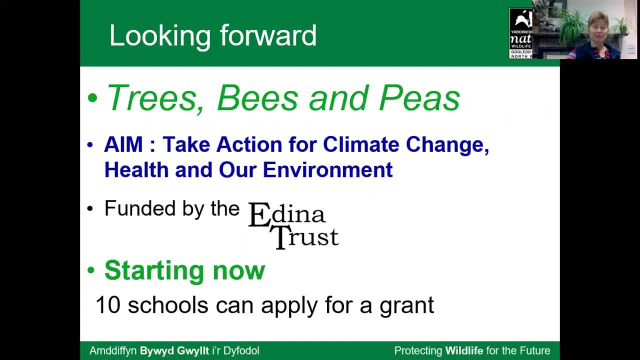 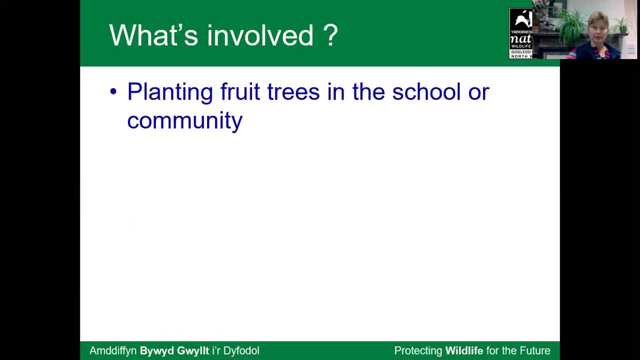 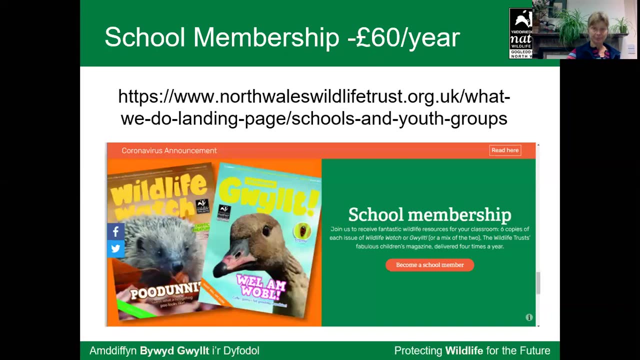 it's both some time for materials at money for materials and some of my time to come and help a project and a half a day of teacher training. so it's about planting fruit trees, hedges, grow veg and a bit of teacher training. the wildlife trust. we also have school membership and you can. 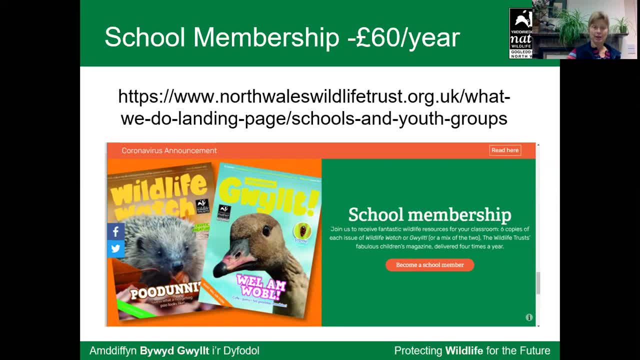 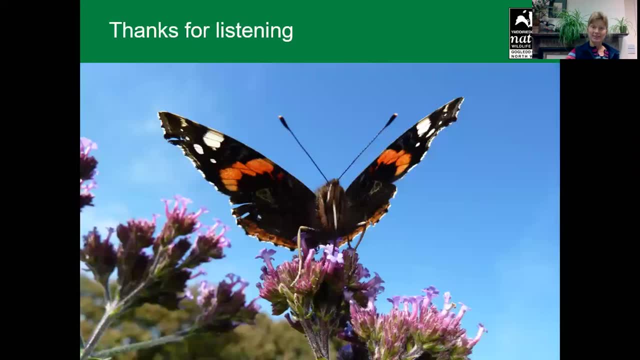 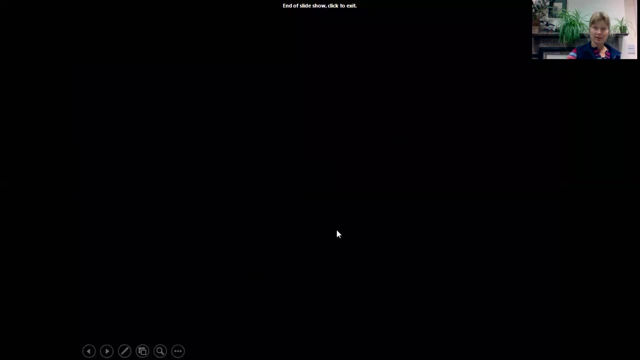 have a look. we'll send you the link and through that you get these magazines which are very popular with children, and also you can access a lot of resources. thank you very much for listening. I'm going to stop talking and if we can all unmute ourselves, then we can have a conversation and you can ask me questions.